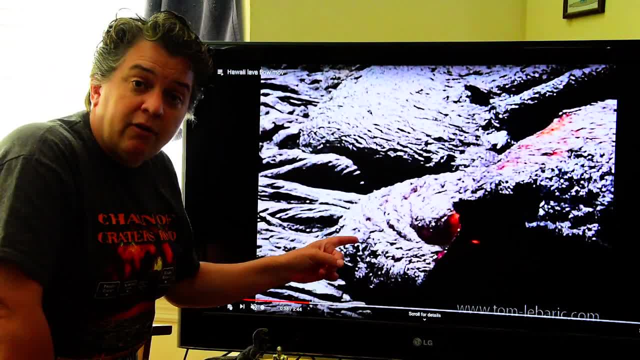 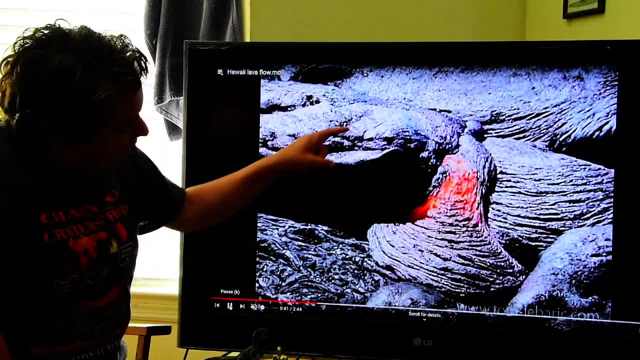 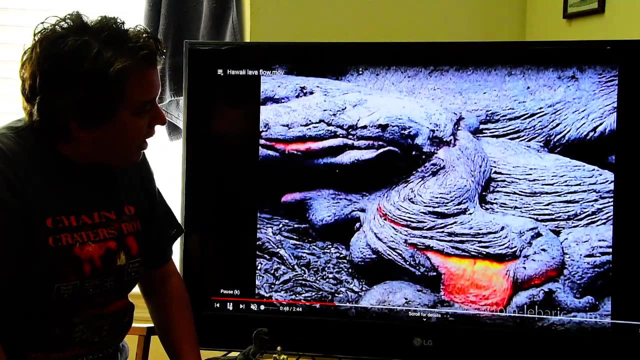 All right, so welcome back to part two. Now we're going to take a look at pohoihoi in action as it forms. So what we're seeing here, these are lava flows in Hawaii, and see how the lava keeps flowing, but the top starts getting wrinkled as it flows there. 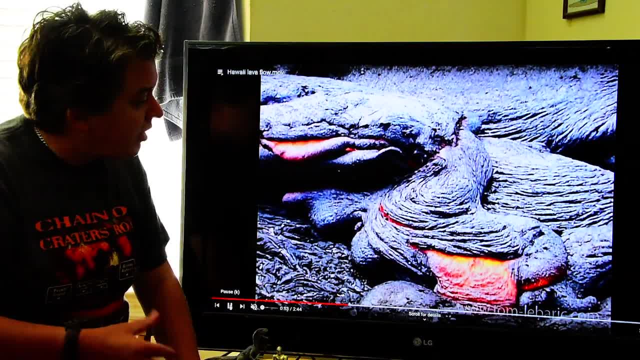 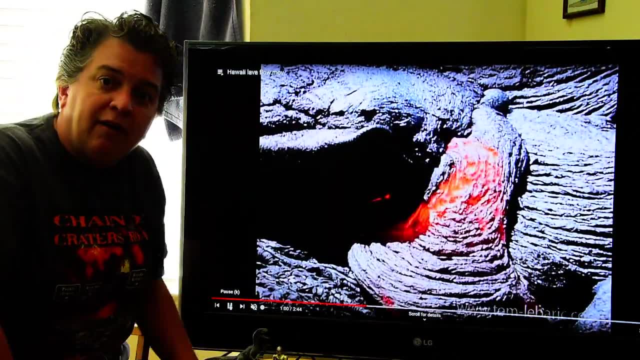 And that's classic pohoihoi formation and ultimately, all that is going to cool down, become solid and preserve this wrinkly lava surface. That's pohoihoi. Let's take a look at ah-ah next. 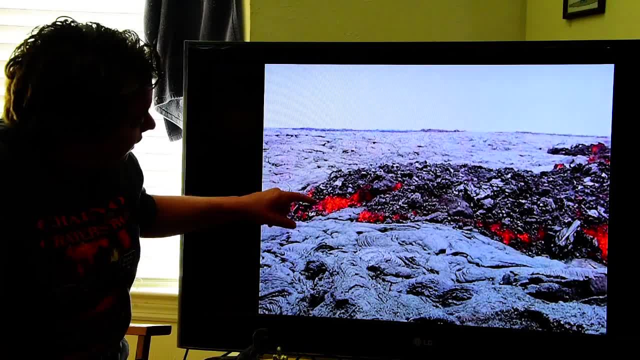 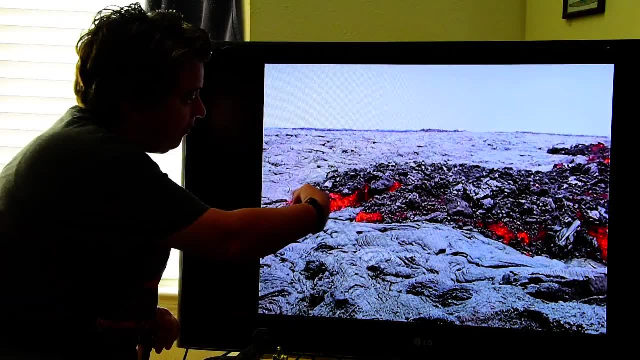 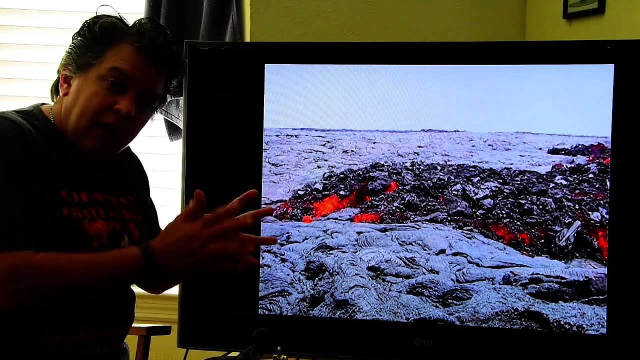 So here we are. Here we have ah-ah flowing. We can see the glowing interior of that lava flow and you can see it's moving very slowly in this direction. This is also in Hawaii and as this cools and contracts gets smaller, you see these chunks falling off. 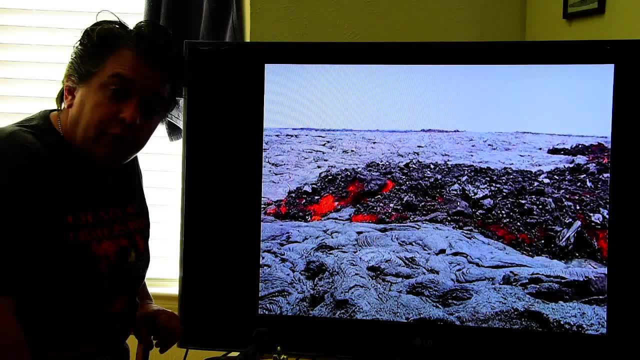 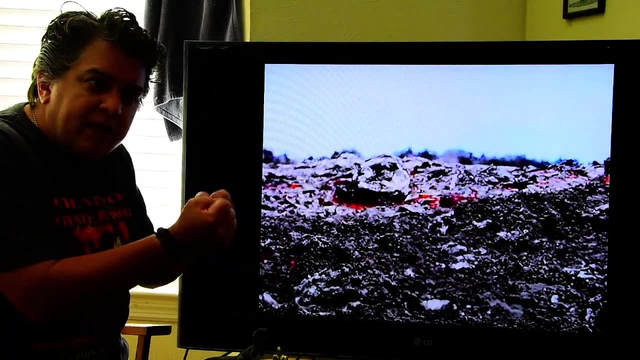 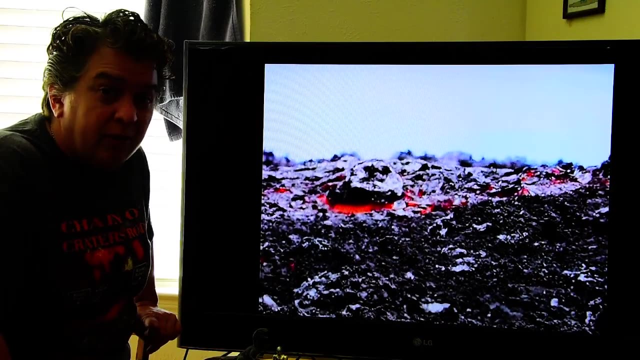 There was a big one that fell off, ultimately creating that very jagged angular surface Of all those pieces that broke off as this lava flow cooled. That's ah-ah, You can walk right up to it. It's hot, though. 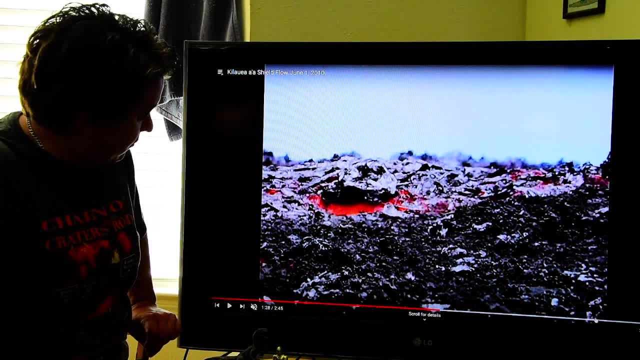 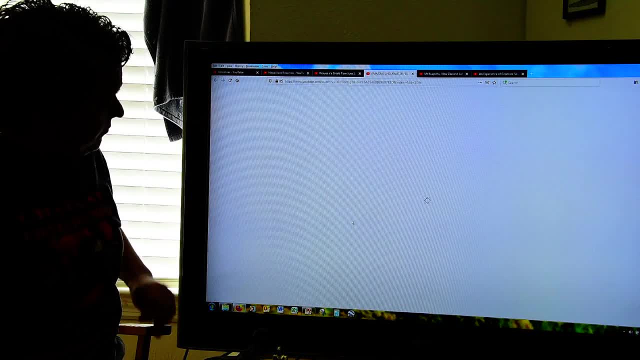 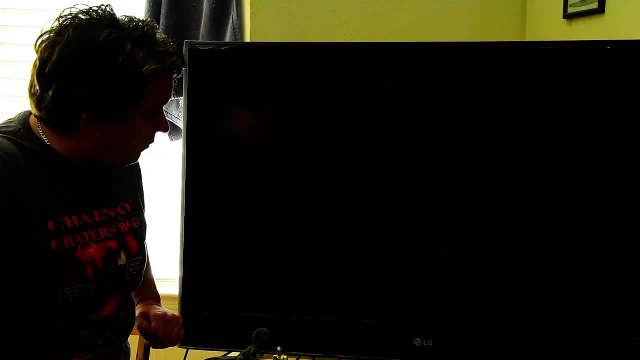 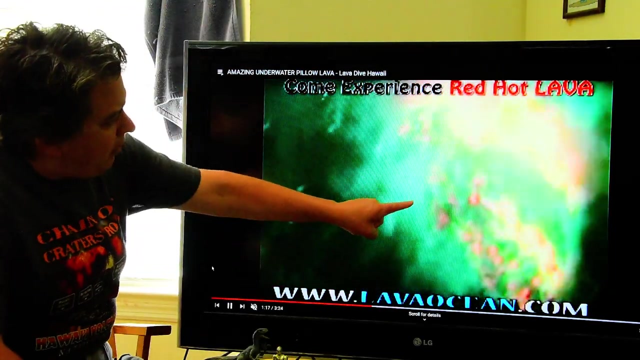 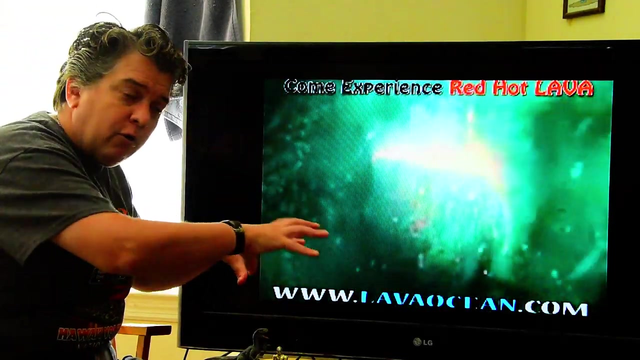 Now let's take a look at pillows. Now we're going to go underwater off the coast of Hawaii, And So here we are underwater and there is the lava coming out. You can see this rounded shape gets cooled, but then more lava flows and another rounded shape comes out. 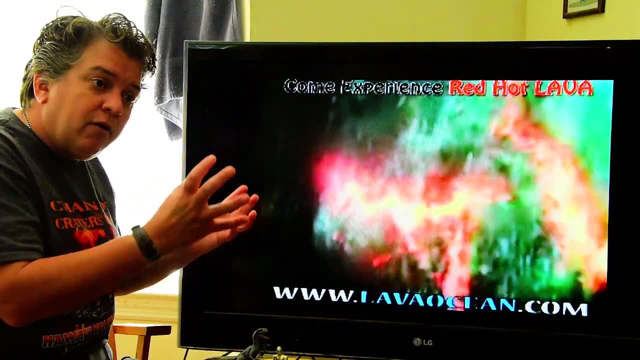 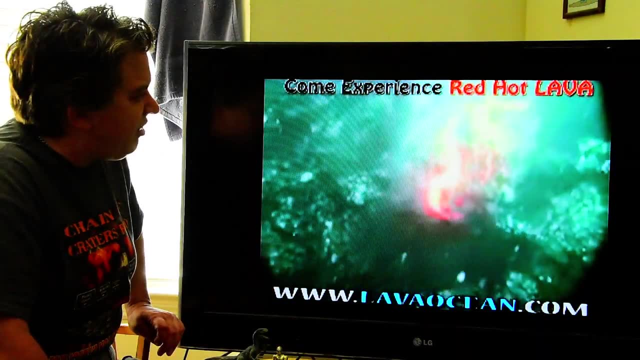 And then more is going to come out and that's how you get all of those rounded shapes of the classic pillow lavas. I always thought it looks kind of like- I don't know- a scene out of Aliens or something like that. 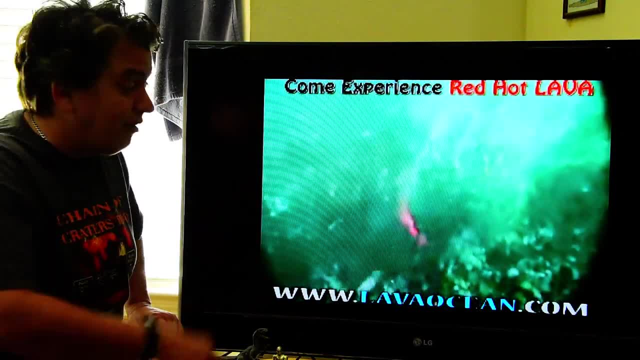 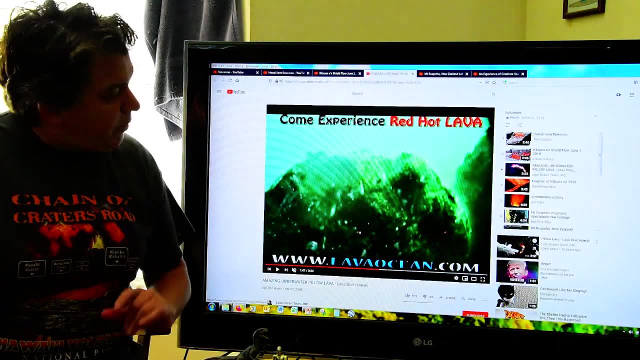 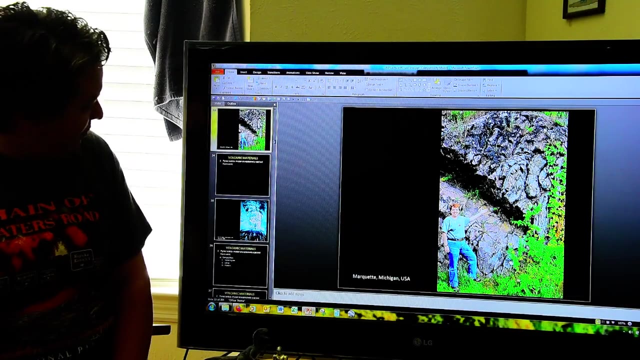 Um, but anyway, Pillow, lavas. So those are some of the shapes that lava can take as it erupts. But when a volcano is, No, not that. yet When a volcano is erupting, we get more than just lava coming out of that volcano. 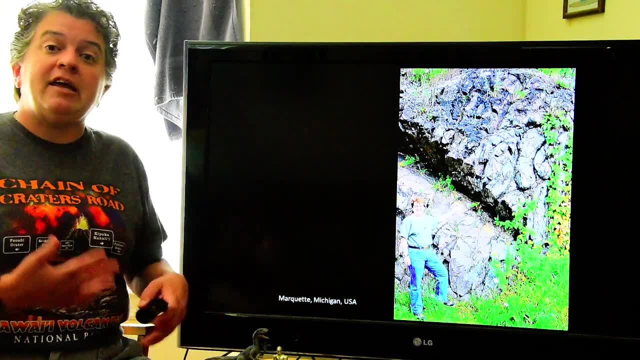 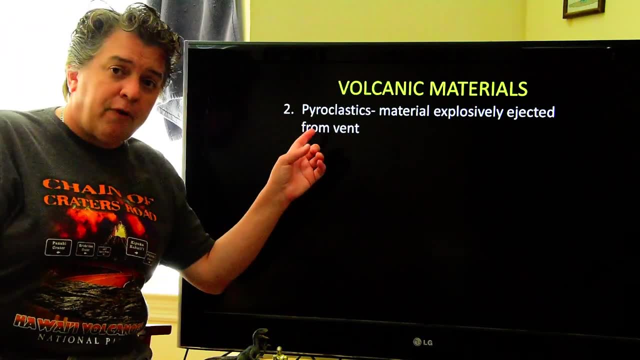 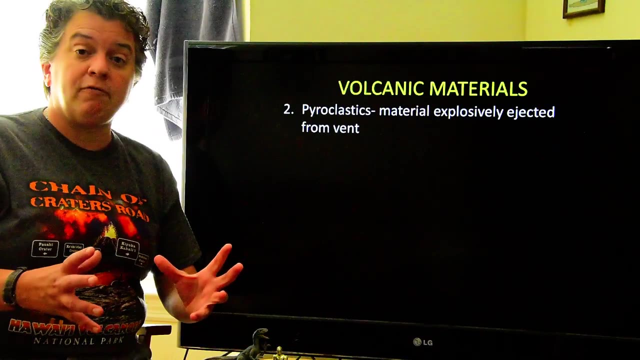 You can get a number of other eruption products Like pyroclastics. Now, the word pyroclastic comes from the Greek. Pyro means fire, Clostos means broken, So this literally means broken fire, And that's because this stuff is. 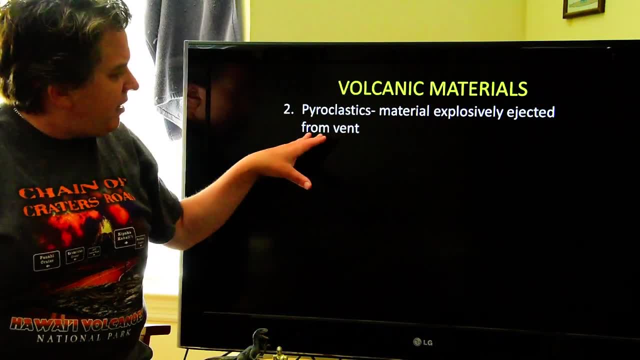 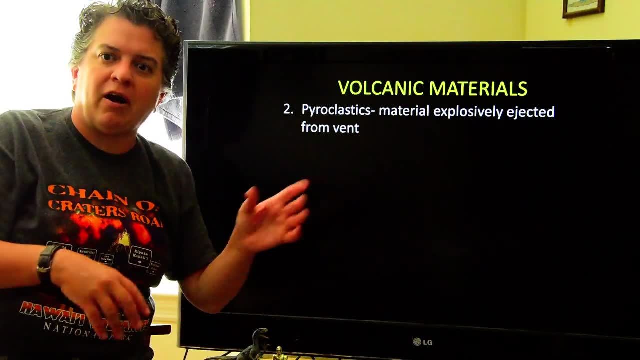 It explodes out of the volcano. And when we say the vent, the vent is basically where whatever is coming out of the volcano is coming out. Okay so volcanic vents where the lava, the pyroclastics, whatever shoots out of the ground. 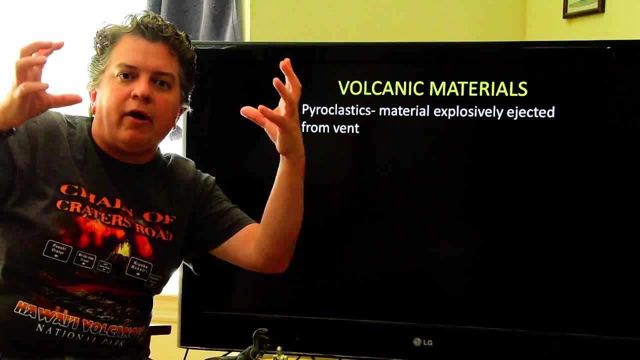 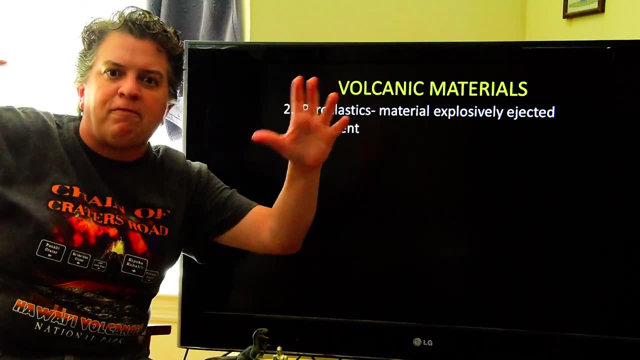 So these pyroclastics explode out of the ground And they're still glowing red hot when they come out of the ground, And so it actually literally looks like broken little bits and pieces of fire flying through the air. That's where they get their name from. 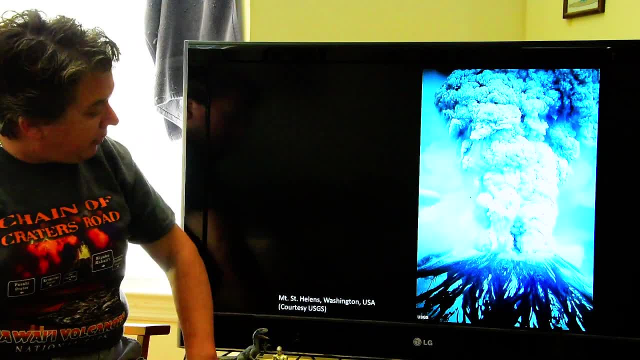 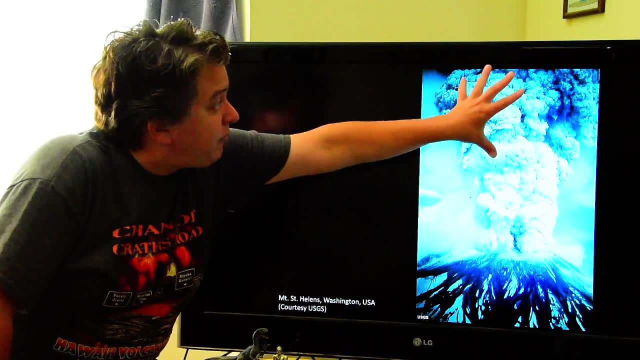 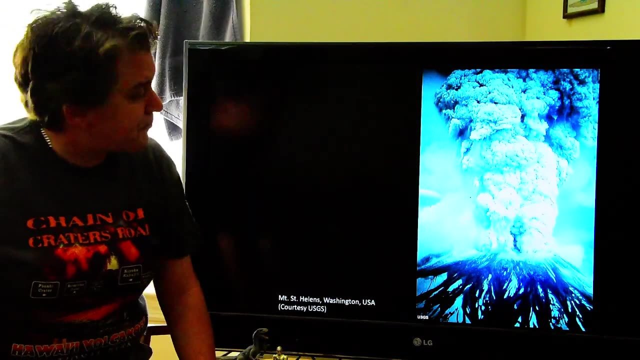 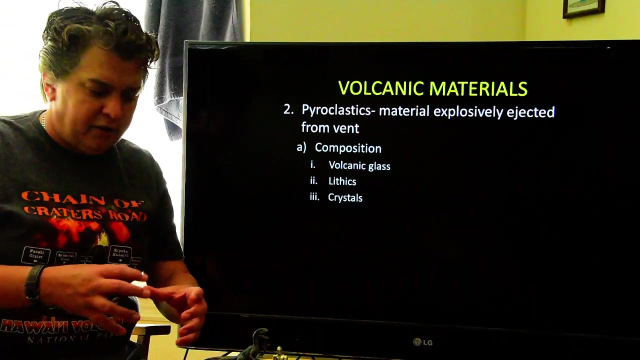 So, um, When you see, like Mount St Helens in 1980, erupting, there's the vent And all of this material is pyroclastic material as well as hot volcanic gases. Now, what would have been in that cloud of pyroclastics? 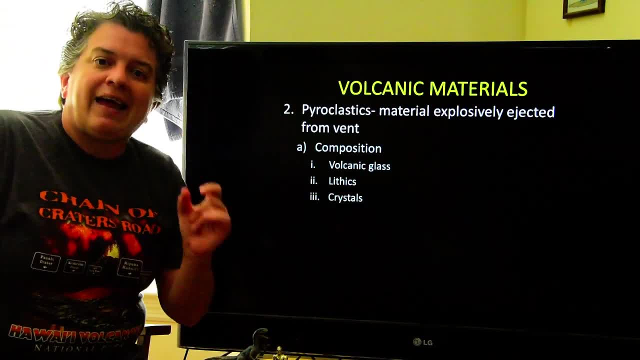 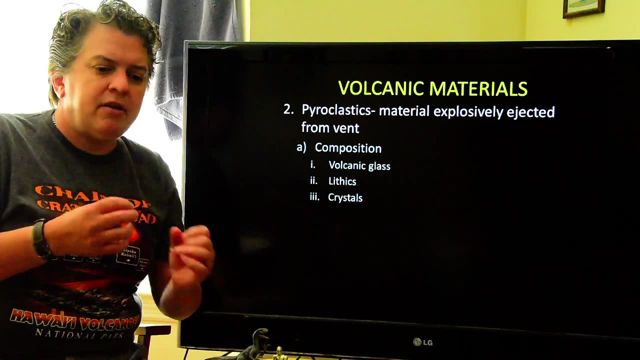 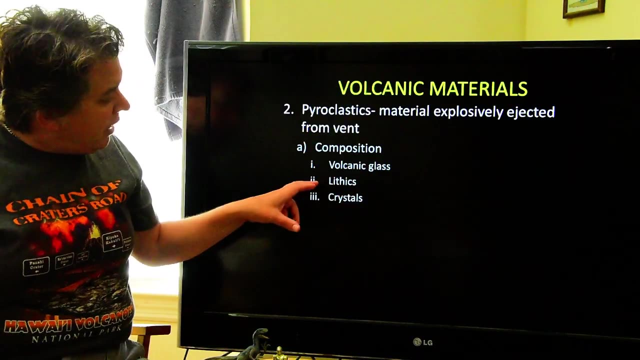 So what are pyroclastics? It's going to be volcanic glass, And volcanic glass is simply basically magma that cooled so quickly it didn't form any crystals, or so It formed just very sharp little jagged shards of glass. There's going to be things called lithics. 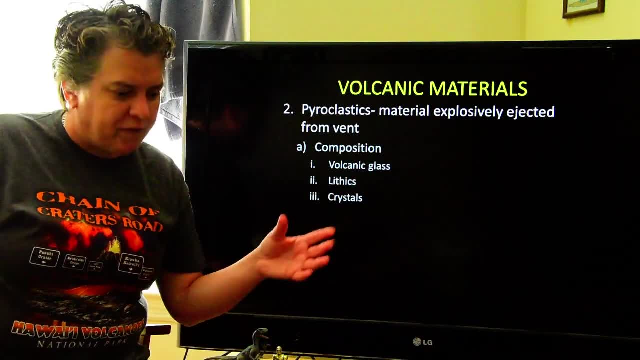 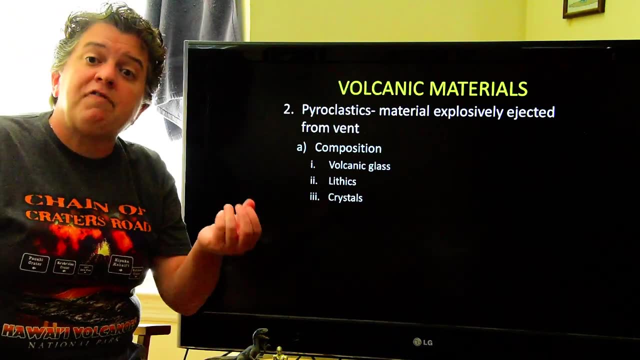 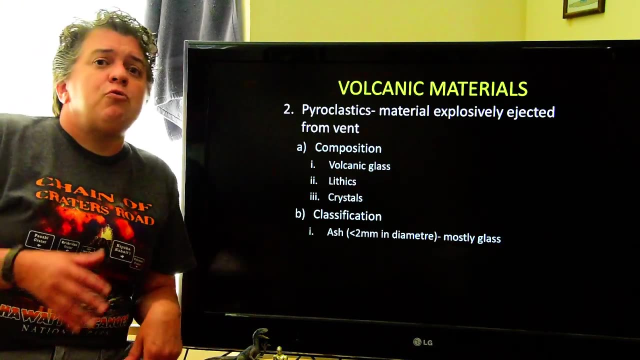 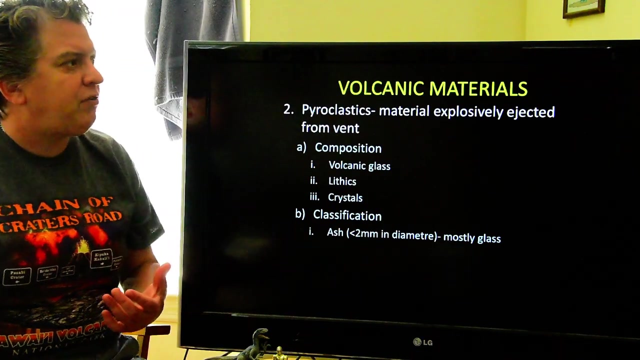 Lithics- are just pieces of rock, solid rock, that just got melted, Caught up in the volcanic explosion. And then there'll also be some crystals, Some minerals that did have enough time to cool before being erupted. Now, when it comes to classifying the pyroclastic material, we look at the size of this material. 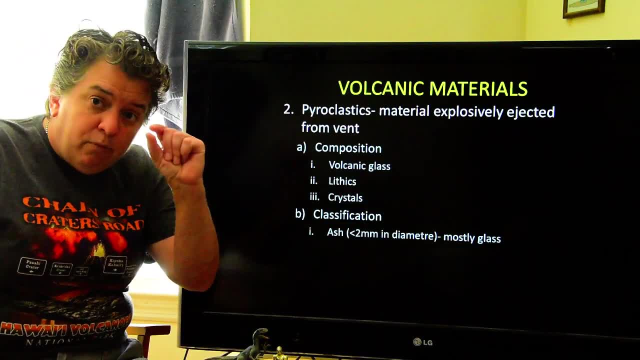 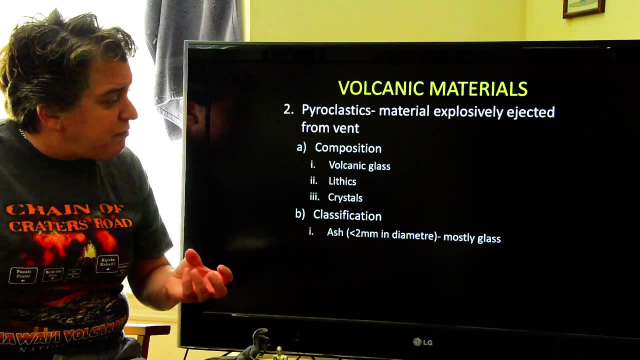 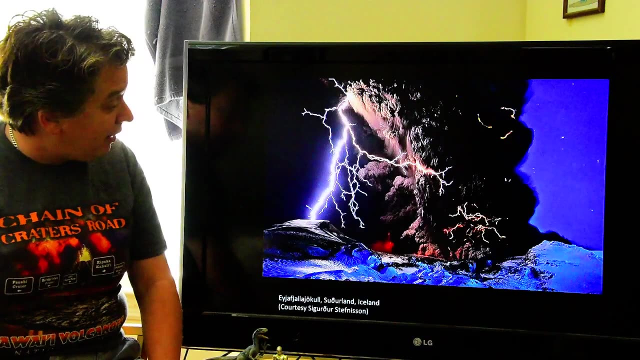 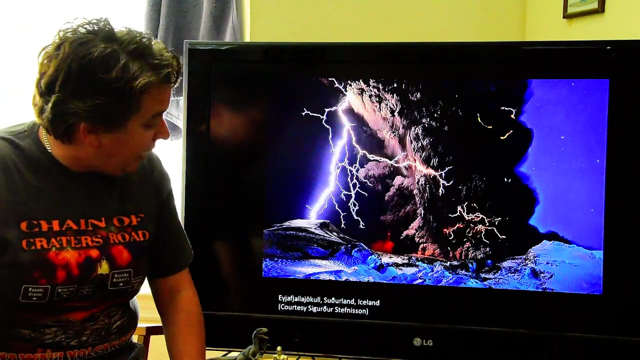 And the smallest stuff, less than 2 millimeters in diameter, usually very powdery in fact, is called ash, And ash is mostly just tiny, almost microscopic pieces of glass- volcanic glass- And this is ash being erupted out of the Icelandic volcano Eyjafjallajökull. 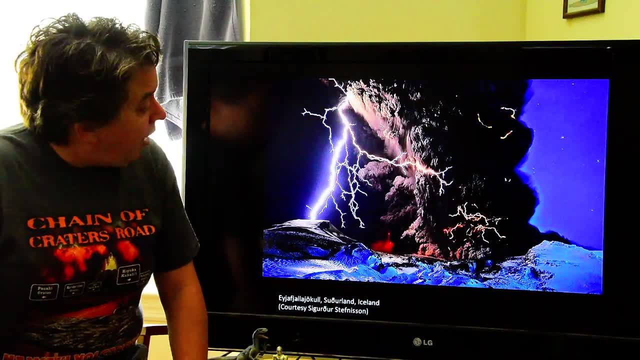 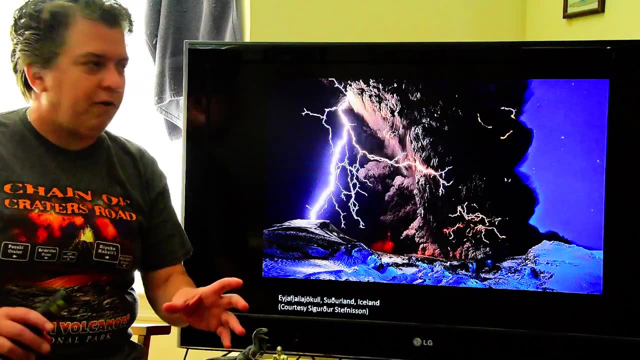 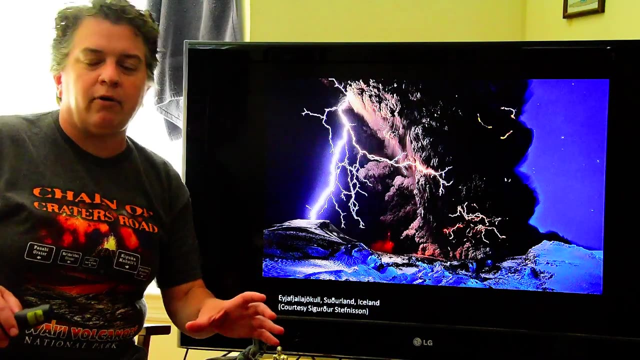 I actually like to show this picture just because it's really pretty. But in addition to that, if you watch these Hollywood movies of volcanic eruptions and stuff, they often put lightning in with it And a lot of my students ask: is that real or is that just to make it look even cooler for Hollywood? 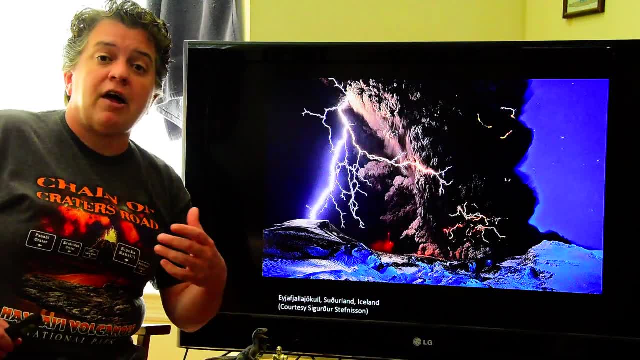 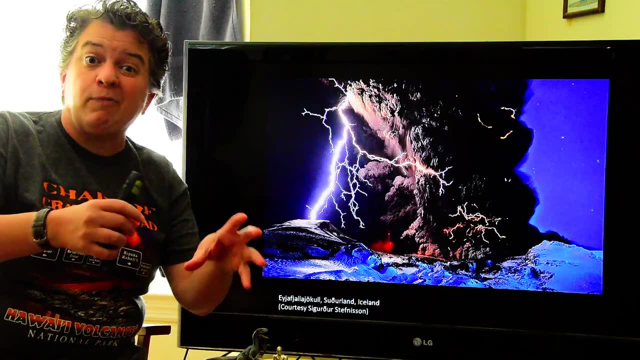 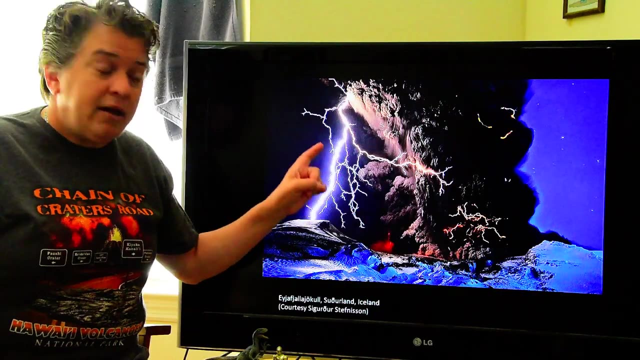 Well, it's real. In volcanic eruptions that have a lot of ash being emitted into the atmosphere, the little ash particles can all rub against each other and build up static electricity, And lightning is a discharge of that static electricity. So in fact, in many volcanic eruptions of this pyroclastic material, 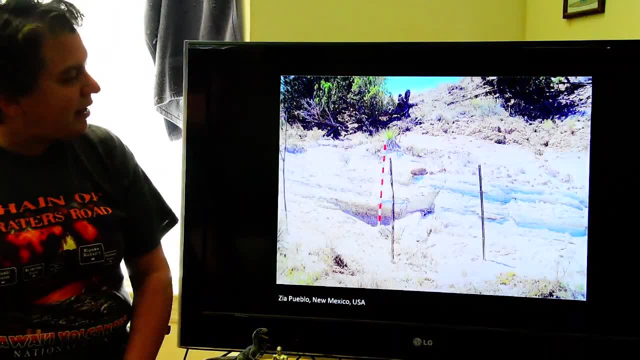 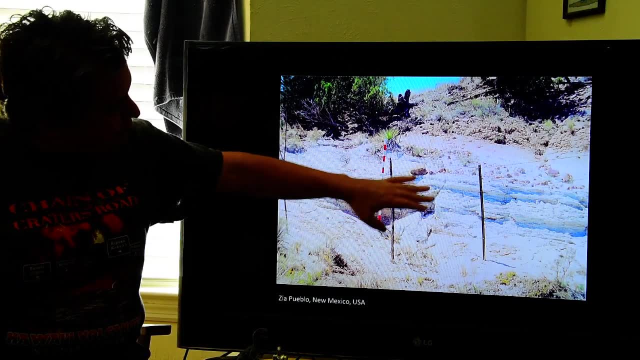 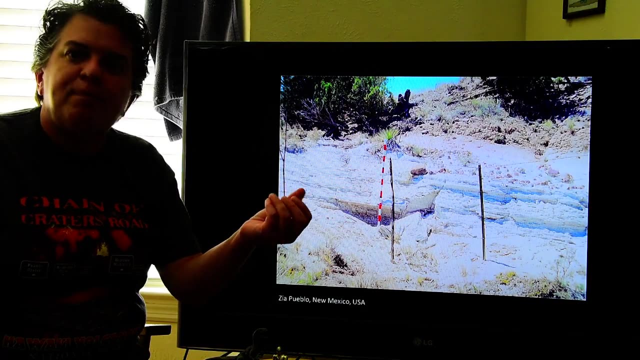 pyroclastic ash. you do get lightning. Now, when that ash lands, if it has cooled in the atmosphere and it lands, it might form a layer like this white stuff you see there, And if you walk up to that you can like poke it and it's very powdery. And that's because this traveled actually a few hundred kilometers in the atmosphere before it was deposited. So it was very cold when it got deposited And you get ash like that. But if that volcanic ash is still hot when it lands, the heat will cause those little glass particles to start fusing together and basically melting together. 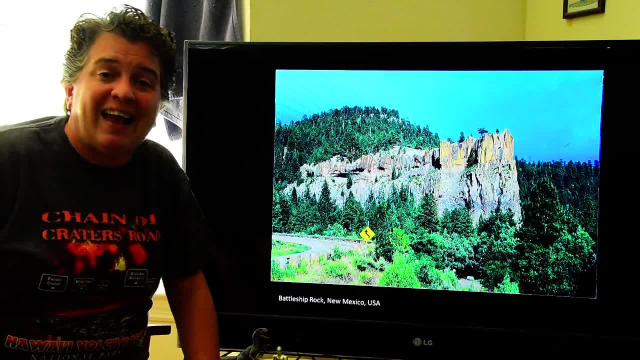 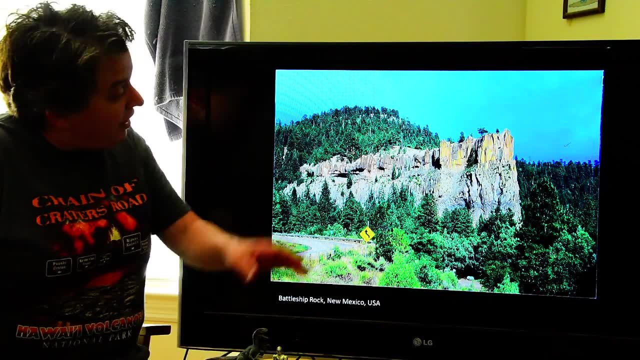 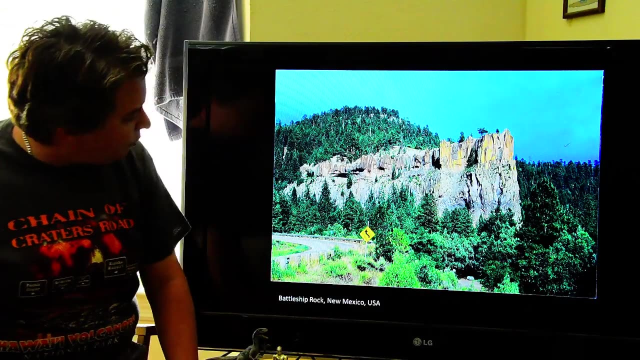 And it will form a rock like this, called volcanic tuff, or we call it welded tuff, And tuff is spelled T-U-F-F, And so that is welded tuff from this ash that landed when it was still hot and it fused together into a rock. 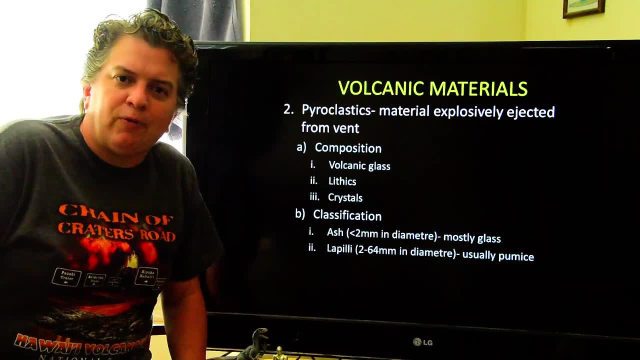 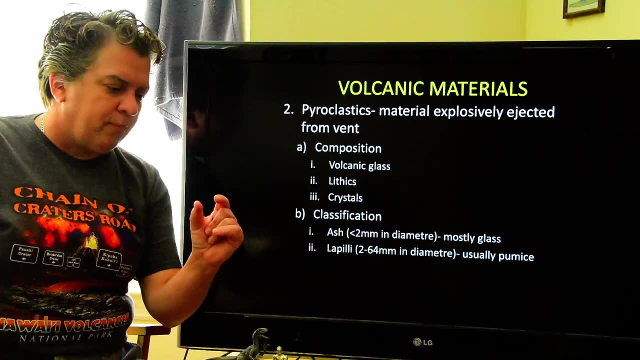 But there's more than just these tiny particles of ash. when we get an eruption of pyroclastics, You also have what are called lapilli. Lapilli are 2 to 64 millimeters in diameter, So they're usually about this size. 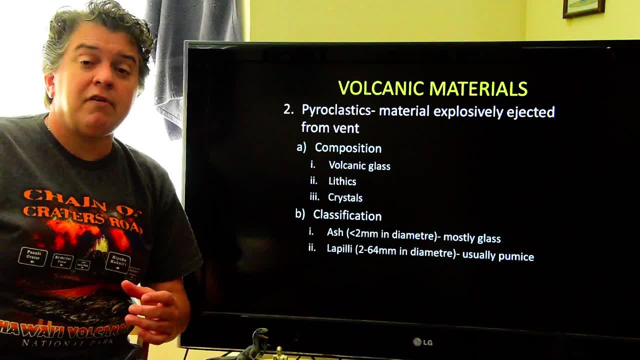 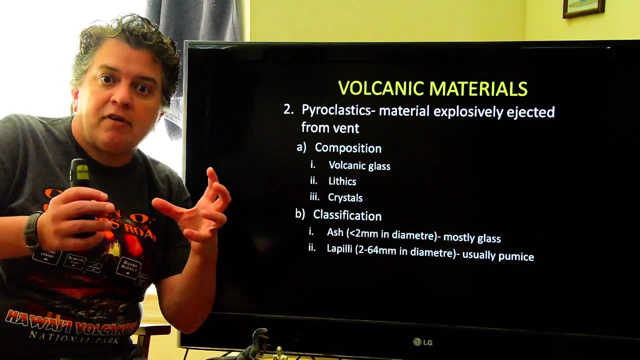 And they're usually pieces of pumice. Pumice is a neat rock because it, in the explosive volcanic eruption, all kinds of little gas bubbles got trapped in it, So it's very lightweight and pumice will float on water. 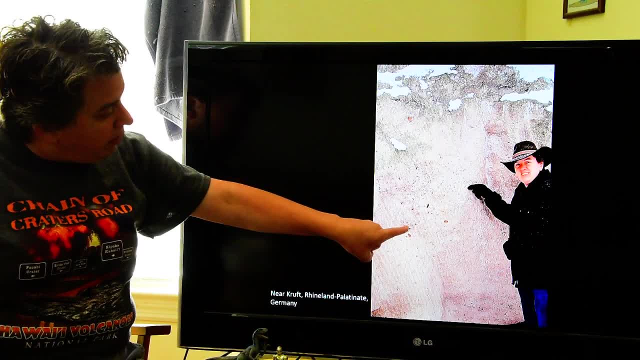 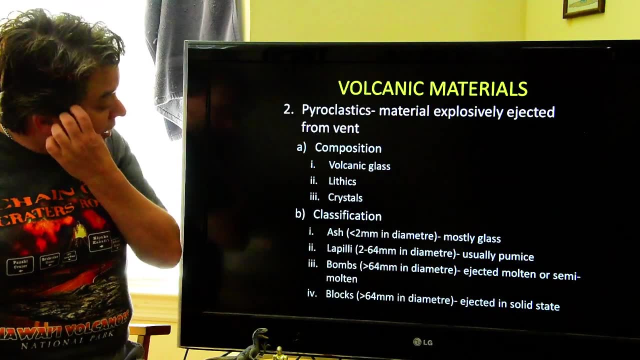 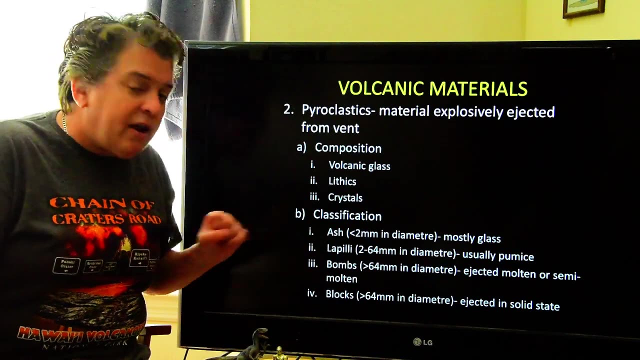 And what we're looking at here. notice all these little fragments in there. Those are lapilli. And then we have the big stuff that gets erupted out of the volcano. We can have bombs and we can have blocks. Both of those are bigger than 64 millimeters. 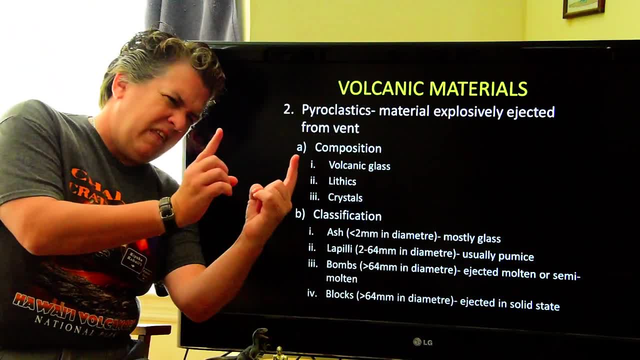 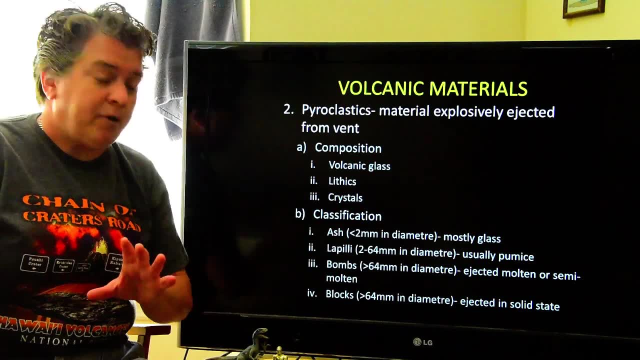 which is like bigger than about that, Maybe that, But anyway these are going to be big objects that get ejected. Now, what's the difference between a bomb and a block? Well, a block when it gets thrown out of the volcano. 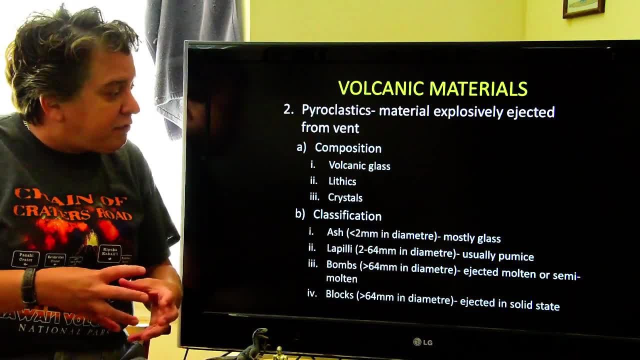 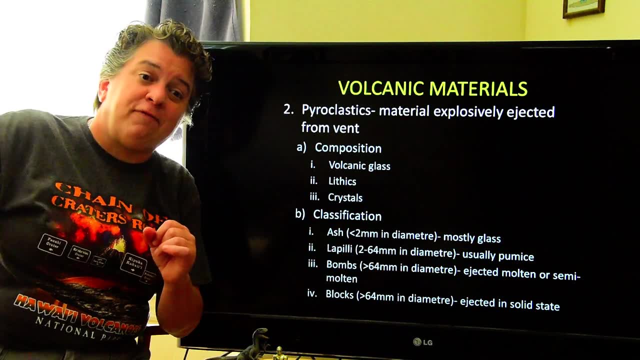 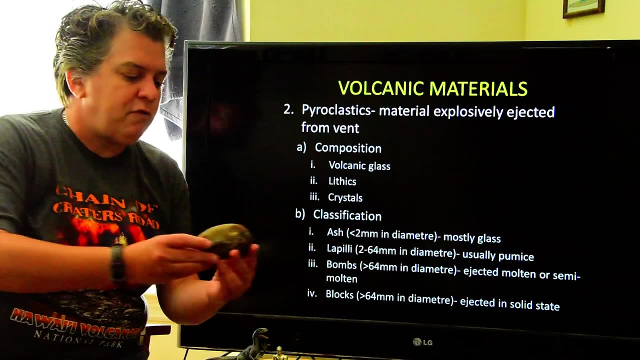 is already solid. A bomb is still molten, or at least semi-molten, So it's at least kind of liquid. So what happens to it? as it's flying through the air, it gets shaped into a teardrop shape. So most volcanic bombs will be like this one right here. 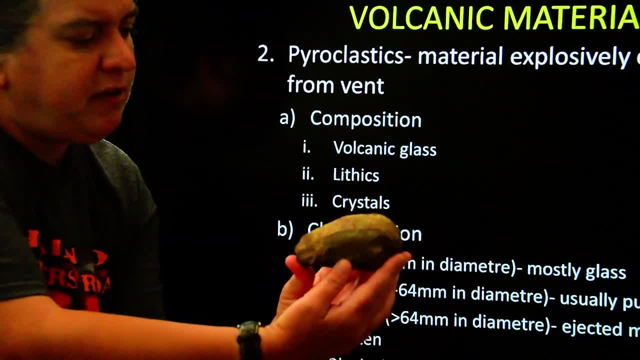 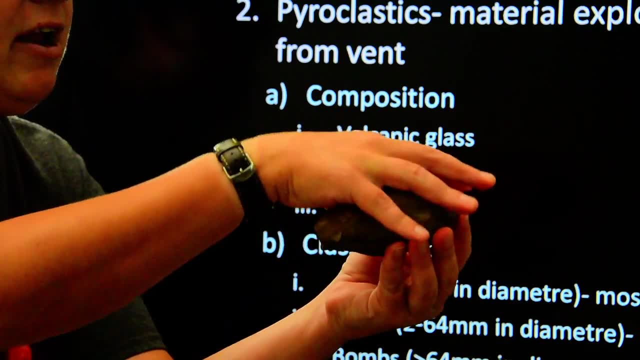 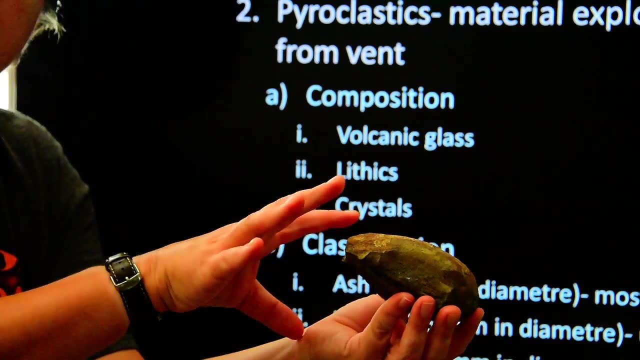 that we have. You can kind of see that, See this teardrop shape to it. That's because this was flying through the air and air resistance shaped that and cooled it. So then, when it landed, it preserved that shape, And this is a very typical shape. 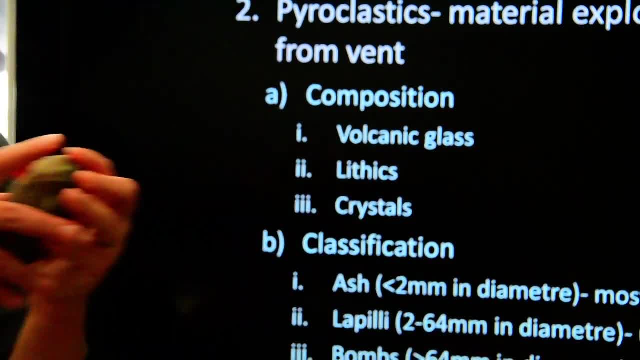 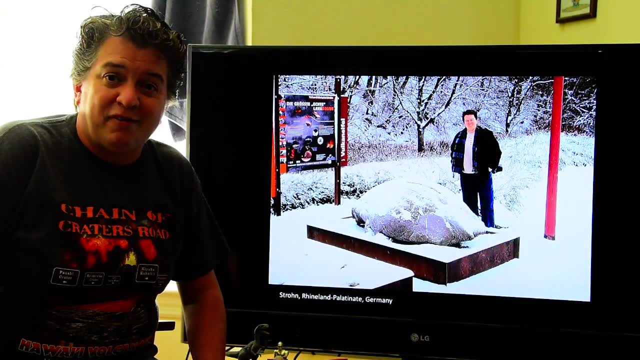 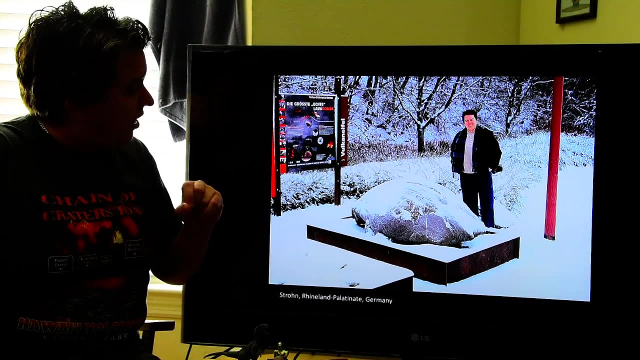 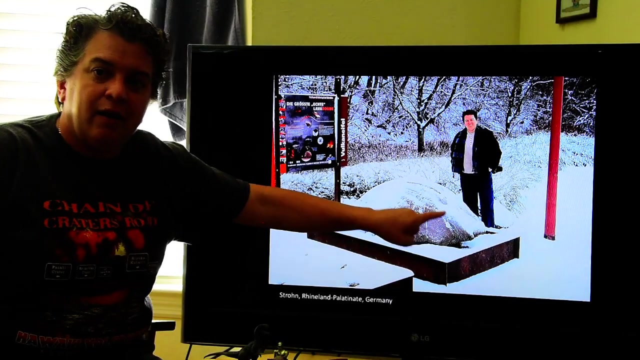 This is the typical size and shape of a volcanic bomb. A not so typical size, but the very typical shape of a volcanic bomb is this one. Now. the sign behind it says the biggest real lava bomb in the world, And you can see it does have that nice aerodynamic shape. 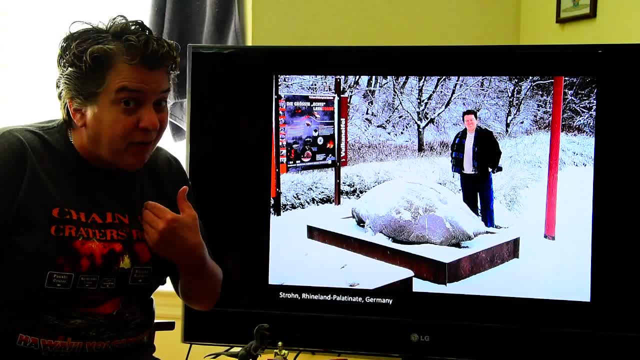 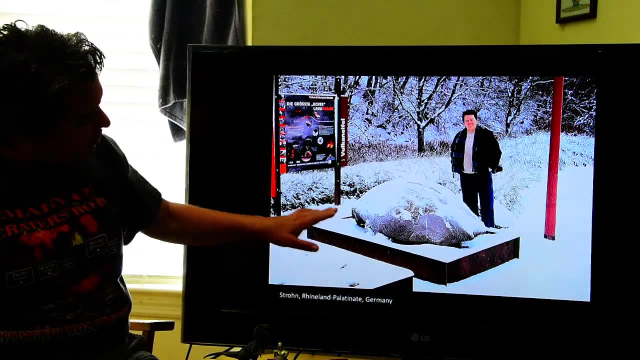 And it is the biggest lava bomb I've ever seen. I can't guarantee that it's the biggest one in the world, but it is the biggest one I've ever seen. But any time you see that aerodynamic shape to these things, that tells you that these were still molten. 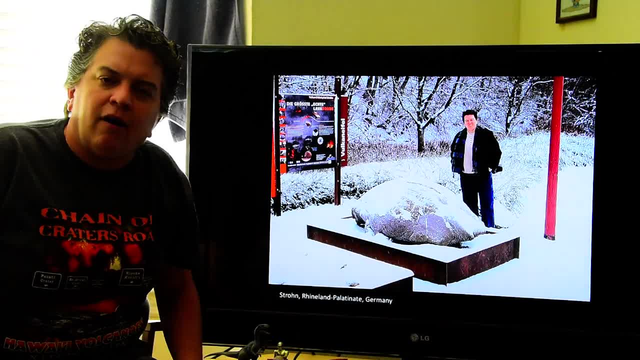 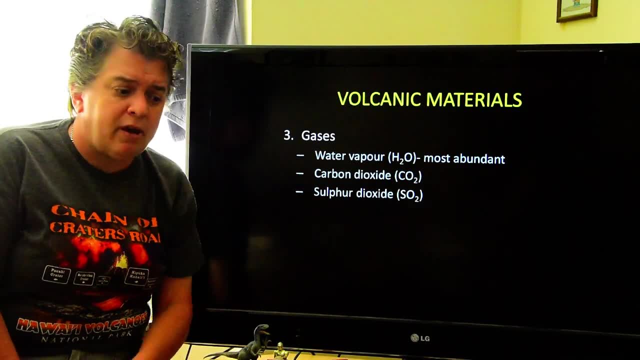 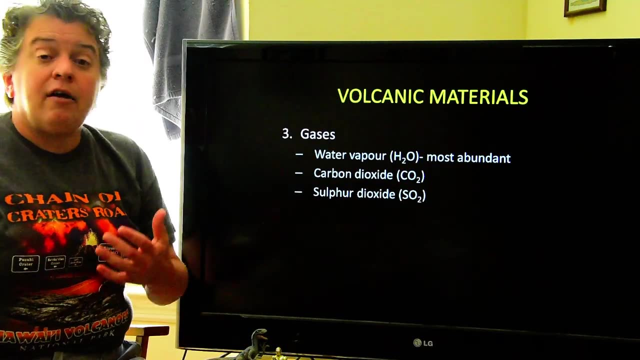 they were still liquid as they're flying through the air out of the volcano. Alright, other things that volcanoes can produce in an eruption- or I shouldn't say can, other things that they will produce are gases, And I already told you. 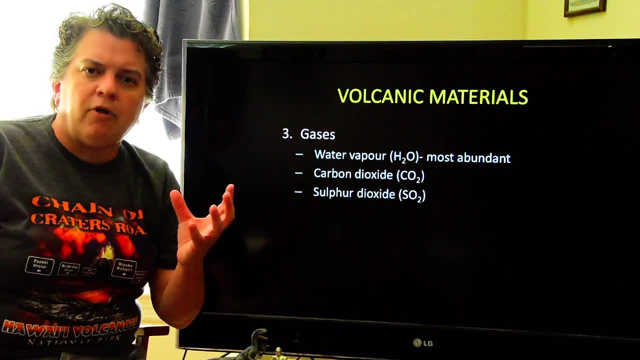 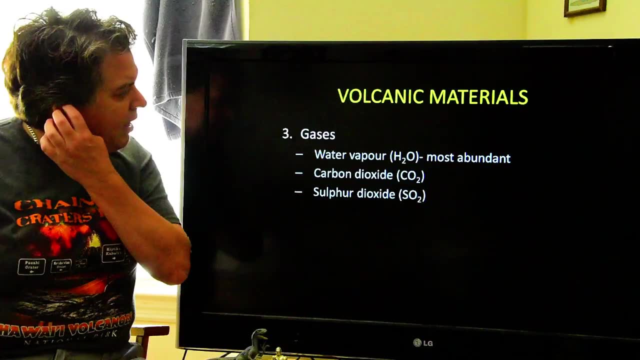 gases are the energy behind the volcanic eruption, right As they expand, as they're rising to the surface. it's that gas pressure that powers the eruption, And there are three main volcanic gases. You have water vapor. this is the most abundant. 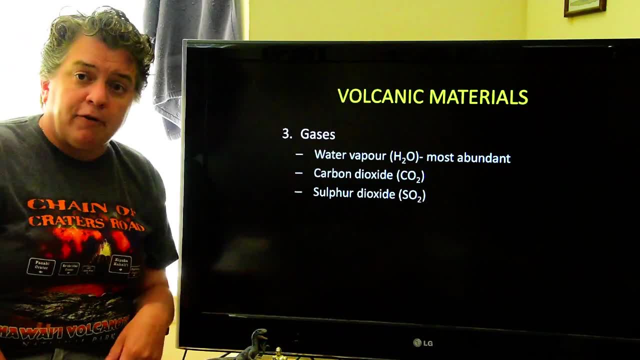 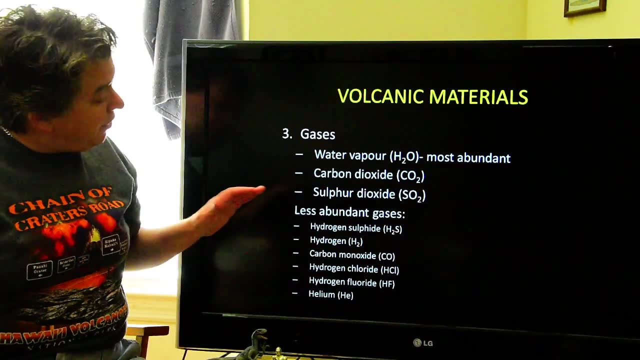 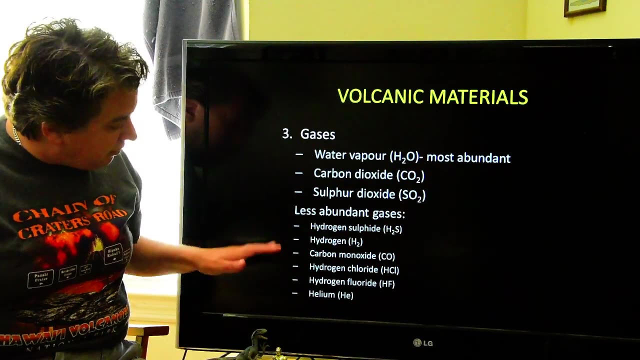 and then you have carbon dioxide and sulfur dioxide. Those are the big three when it comes to volcanic gases. However, there are some less abundant gases like hydrogen sulfide, hydrogen carbon monoxide and some others. Some volcanoes actually give off a fair bit of hydrogen fluoride. 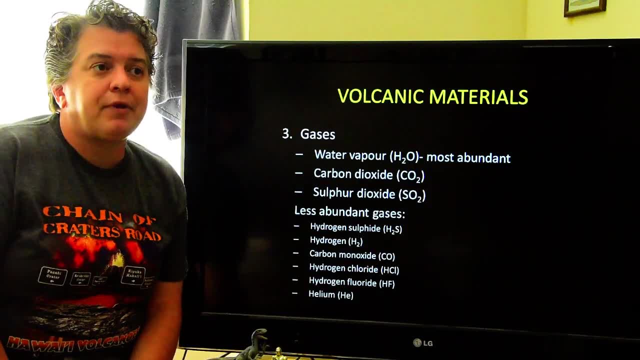 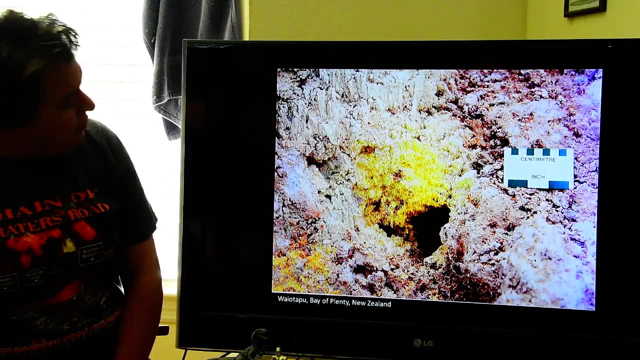 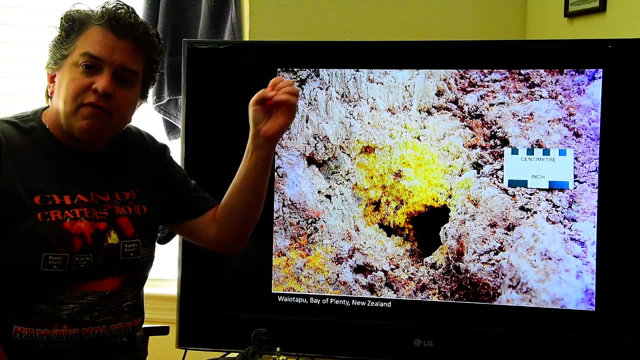 which can cause a deadly disease called fluorosis that we'll talk a little bit about later. This is something known as a fumarole, and a fumarole is where a volcano is giving off. it's venting some of these volcanic gases. 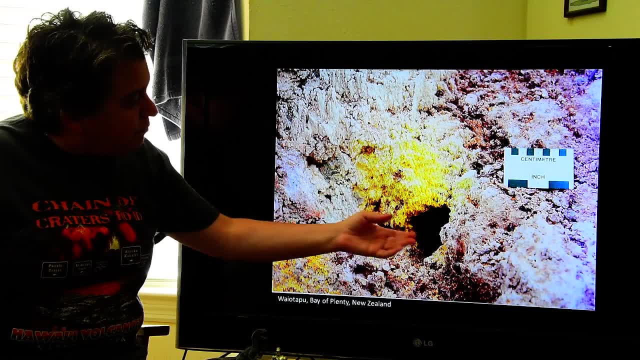 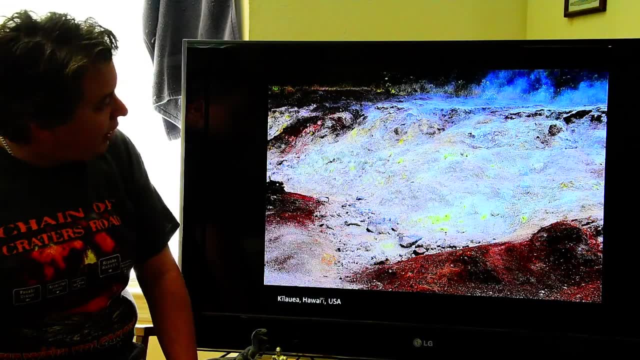 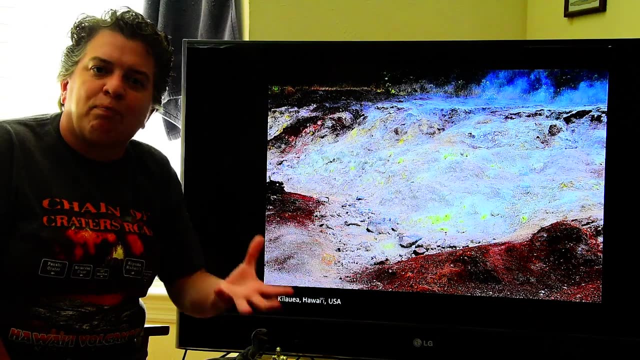 And this happens to be sulfur-rich gas, because as it's coming out of this fumarole right here, it's depositing some crystals of sulfur. We can see the same thing occurring here: All these nice tiny little fumaroles where the volcano is breathing. 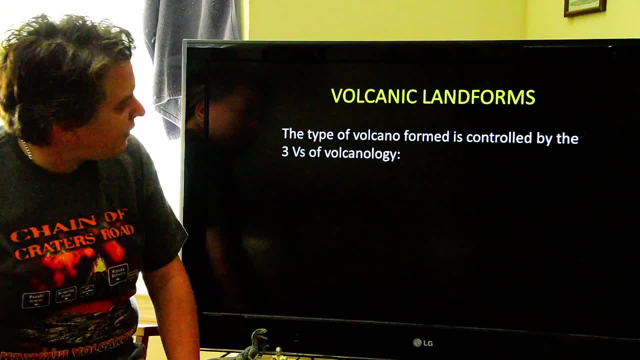 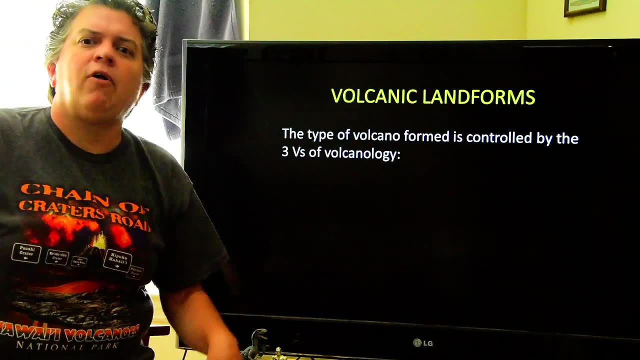 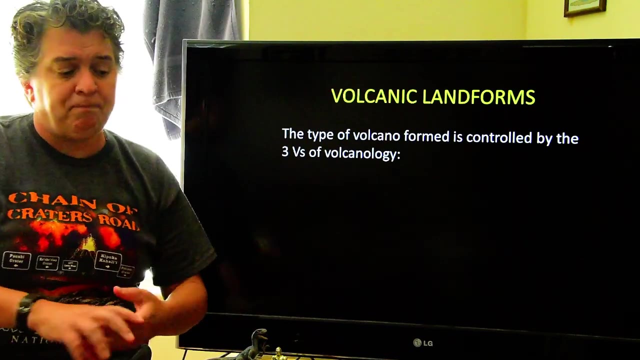 it's giving off some of those gases. Alright, so now we know the things that come out of a volcano when that volcano erupts. We have the lava, we have the pyroclastics and we have the gases Now, as eruptions occur, 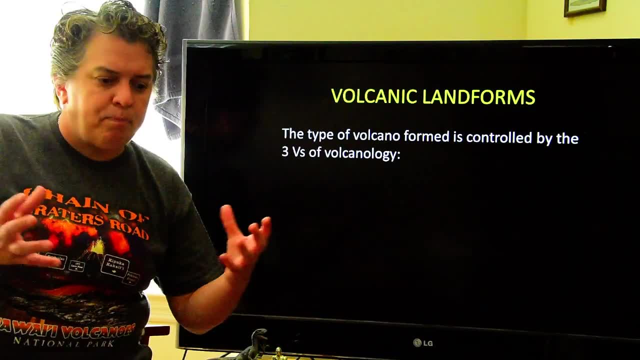 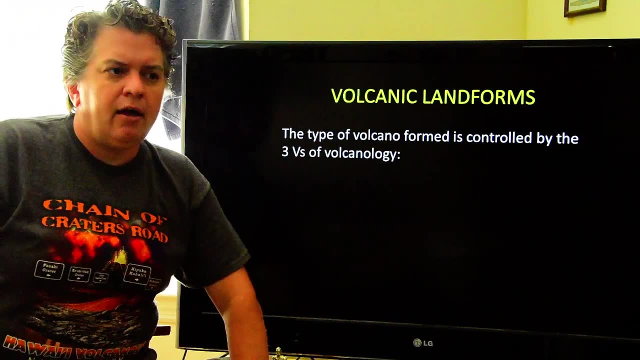 it's going to create a volcanic landform. It's going to build up a volcano And most of the time when I ask people, what's a volcano, look like. You know, if I give like a six-year-old a piece of paper and some crayons, 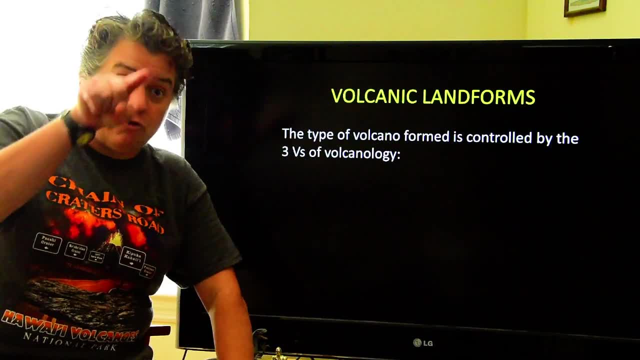 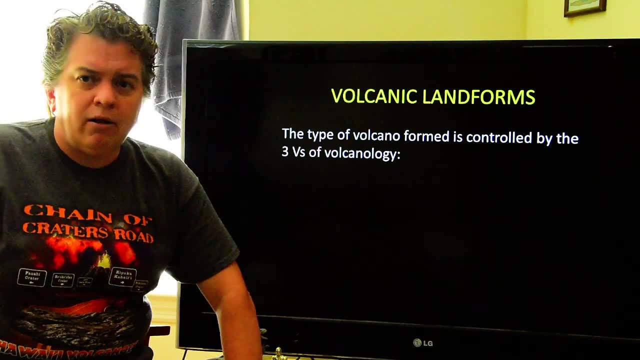 and say: draw a volcano. for me, it's probably going to be a cone-shaped mountain with a crater on top, Because that's what most people picture, basically like Mount Fuji. right, Well, that is a volcano. However, there are many different types of volcanoes. 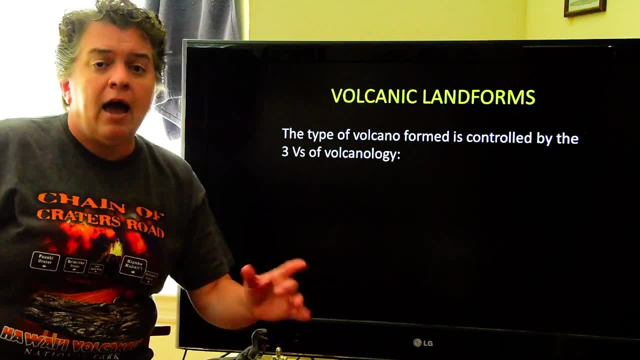 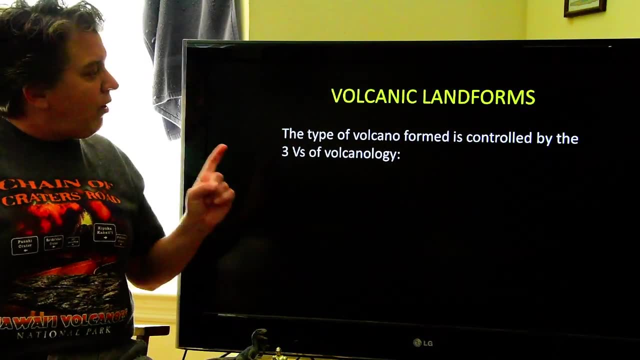 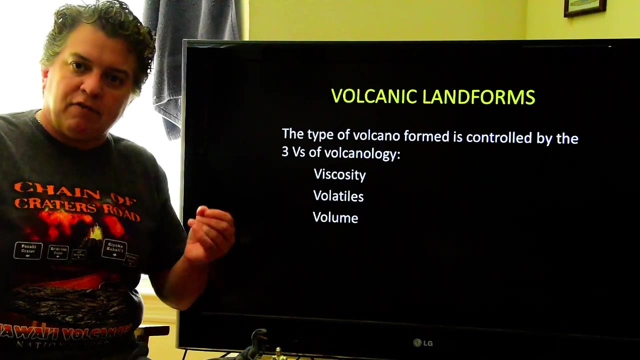 that come in different shapes and sizes. And what controls the shape and the size of the volcanic landform that's created are what we call the three V's of volcanology: Viscosity, that's, the viscosity of the lava coming out. The volatiles- that means 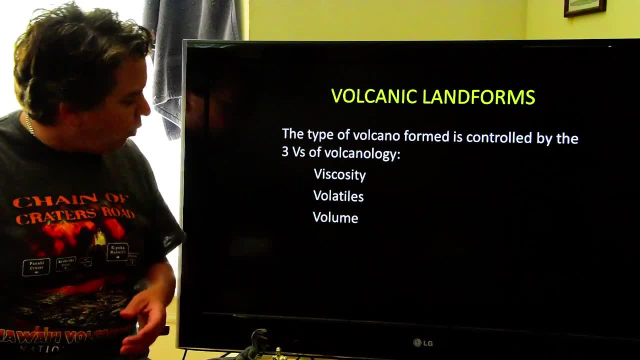 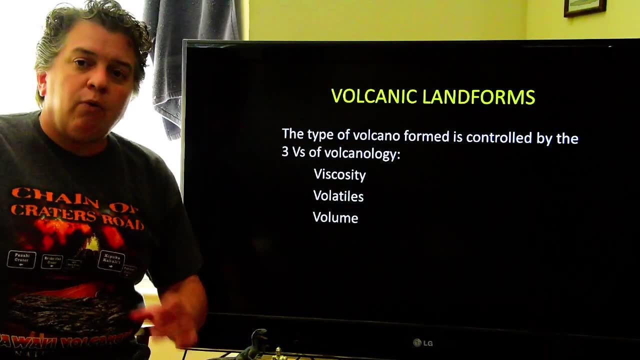 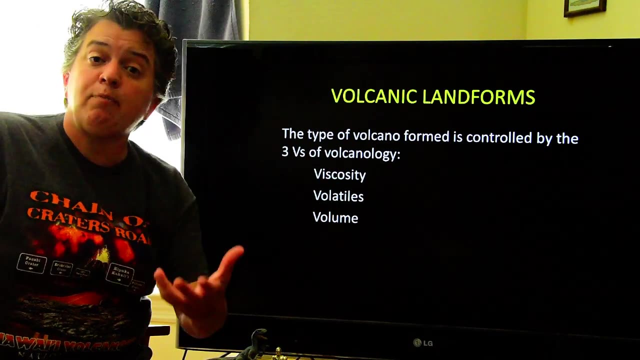 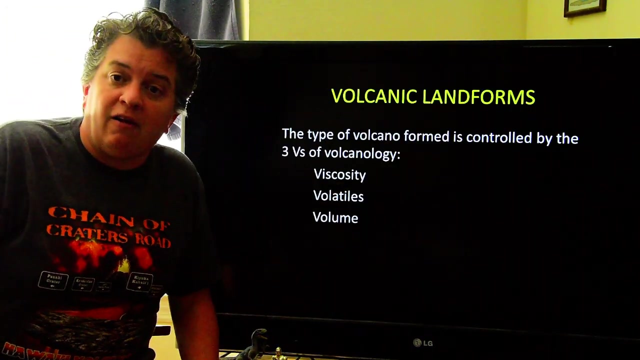 is the lava- gas-rich or gas-poor- And the volume- just how much lava is being erupted. So what we're going to do next is take a look at the different volcanic landforms, basically the different types of volcanoes created, and then see how these three V's of volcanology 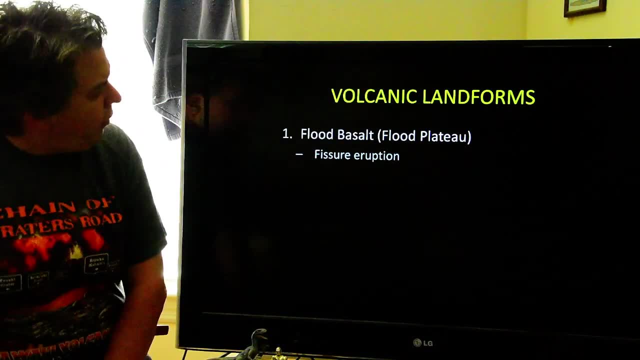 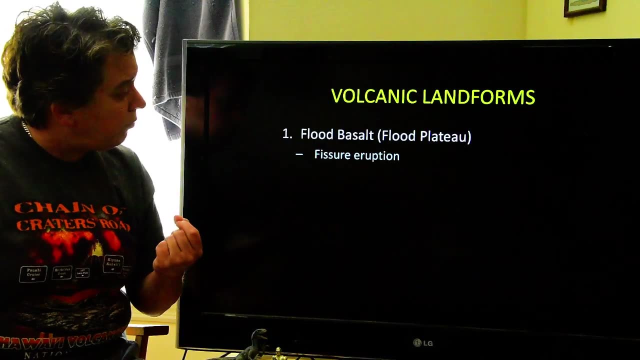 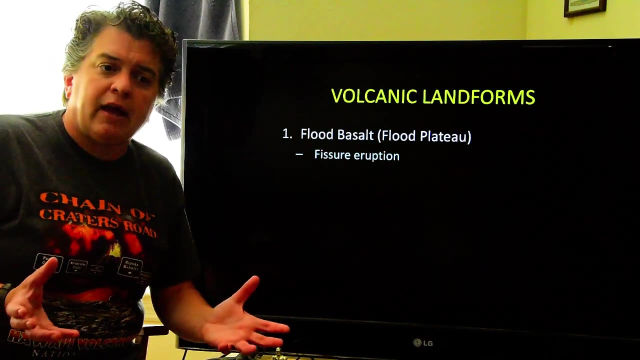 affect their shape. Now we're going to begin with what's called a flood basalt. These also are sometimes called flood plateaus. This comes from a fissure eruption. So first of all, you know, often times when we think of volcanoes, 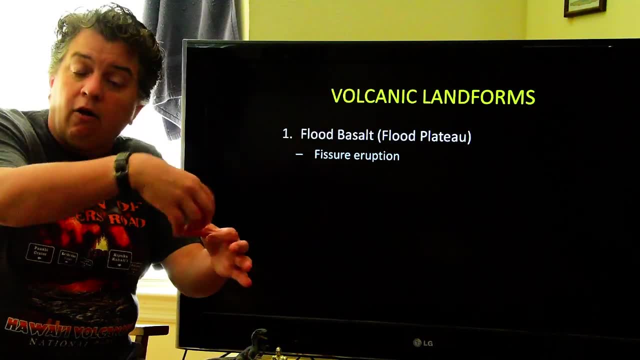 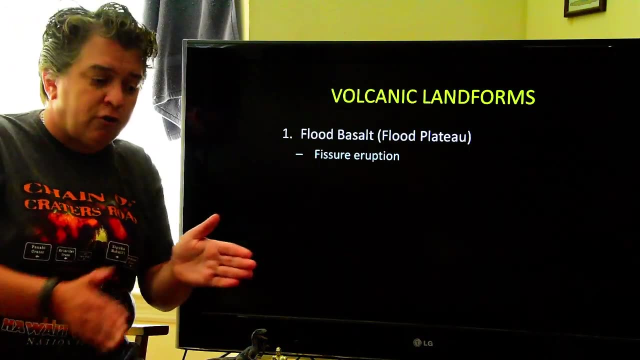 we think that they have this like little central crater where everything, all the lava and stuff, comes out, And that's true for many volcanoes, but not for this In this case. what a fissure is? it's where a big, long crack. 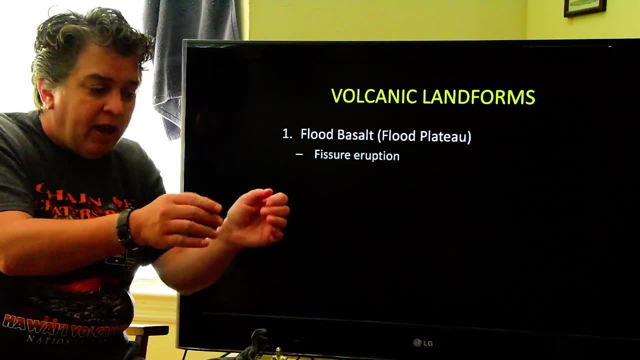 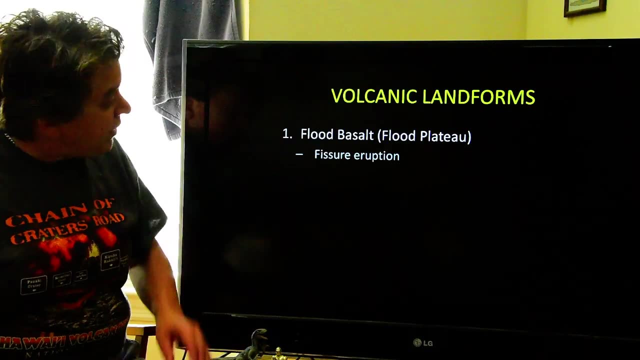 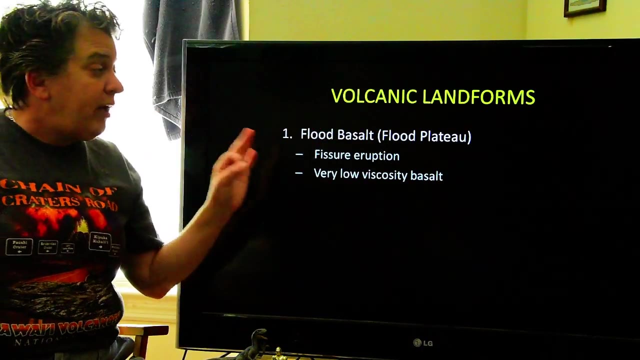 sometimes many kilometers long, opens up and then lava flows to the surface at that crack and then flows around and covers the land around that. So fissure eruption, the vent is not a point. it's a big, long crack Now in flood basalts. 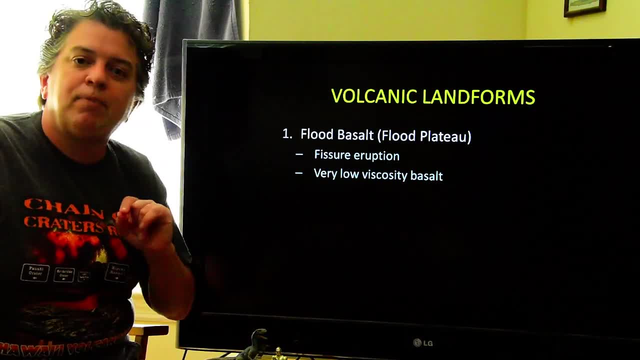 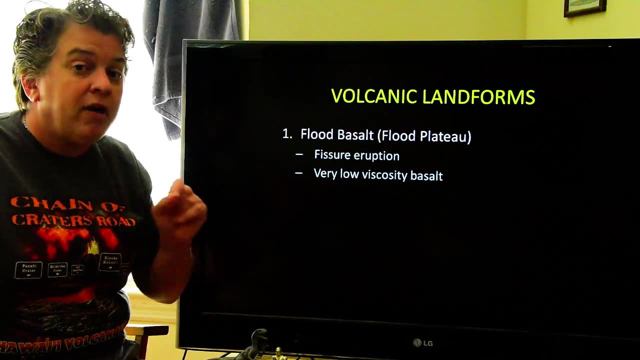 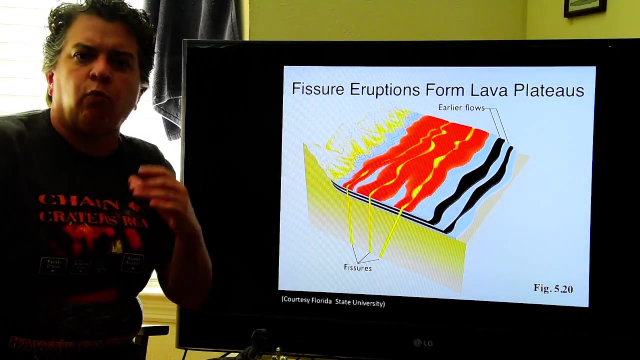 you get very low viscosity basalt. That means the lava can flow a long, long distance from that fissure where it comes from. That's what we're seeing here Now. don't think that this is going to be like one single eruption. 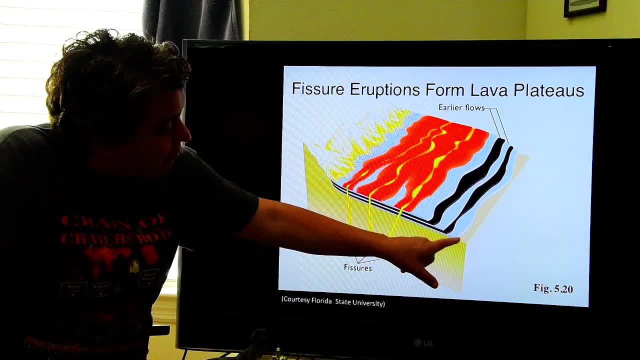 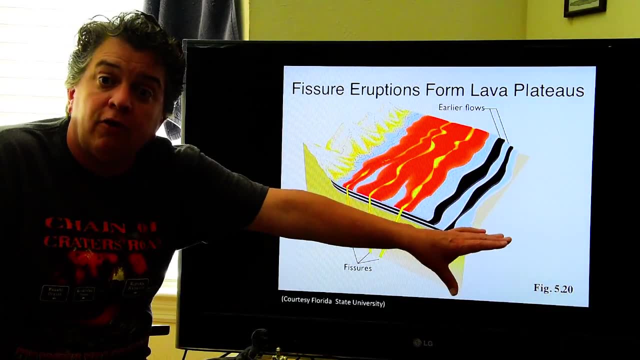 Basically, a fissure will open, a lava flow will flow away from that. it'll cool, it'll become solid. then maybe another fissure opens, another lava flow flows out, cools, crystallizes, becomes solid. So you actually get a whole stack. 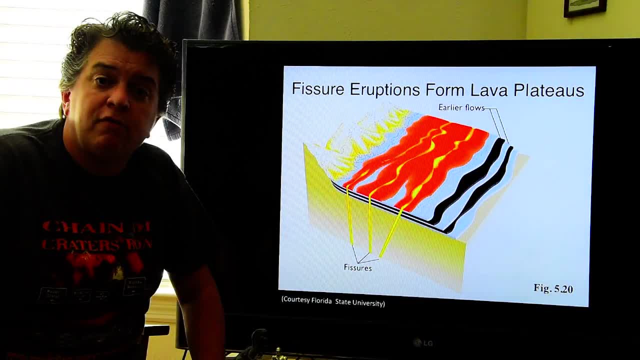 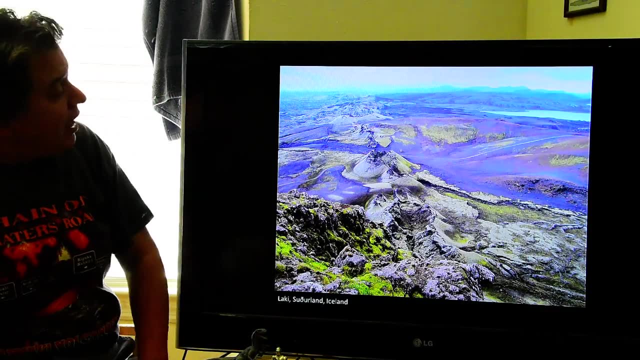 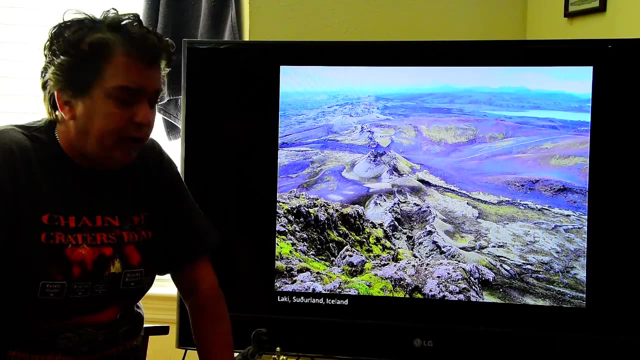 of these lava flows, when you have these fissures of flood basalt eruptions- And that's what we're trying to look at there- And there's that long fissure. The most recent flood basalt eruption that occurred was in 1783. 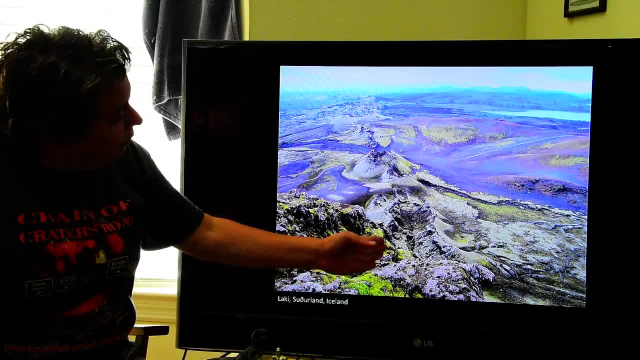 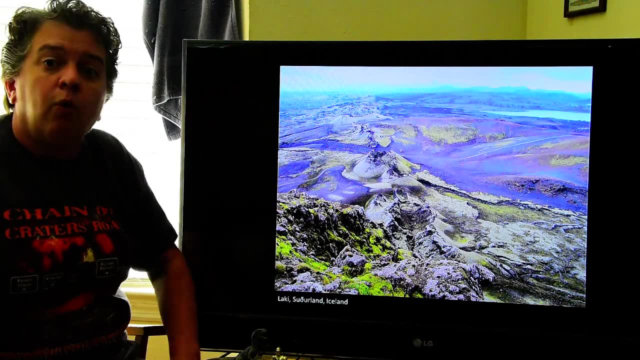 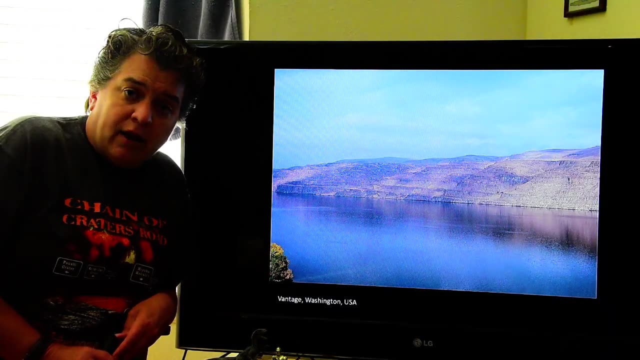 when Laki in Iceland erupted, And we are looking right down that fissure. So this is what opened in 1783, and then lava flowed away from that. We do, however, have flood basalts here in the United States, It's just they're a lot older. 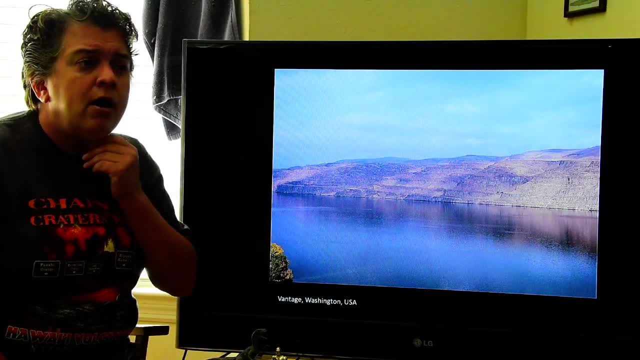 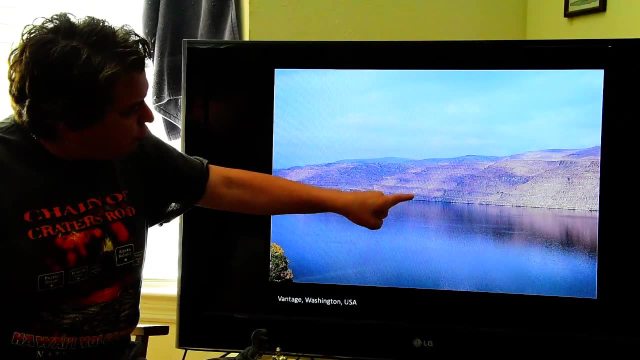 We're looking here at the Columbia River Plateau off in. this is in Washington State, And do you see this kind of stair-step pattern over here? Each one of those steps is a lava flow. These, though, are around 15 million years old. 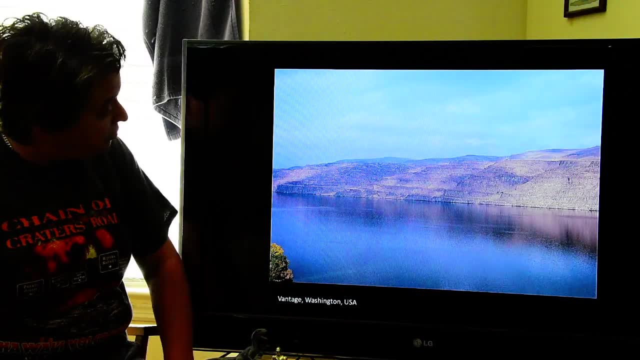 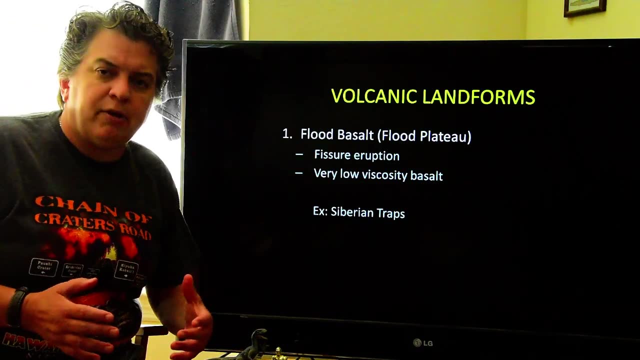 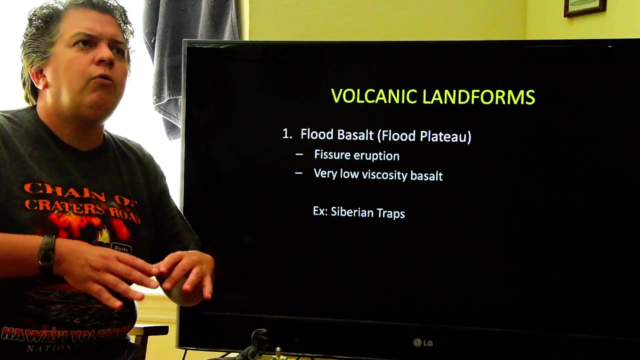 So they're a lot older than the Laki eruption. Now, when I talk about volcanic eruptions, people often ask me, like, what are the biggest eruptions? And that's a hard question to answer, because what are we calling biggest? 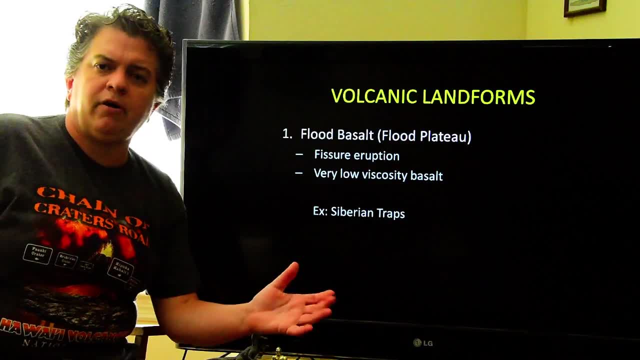 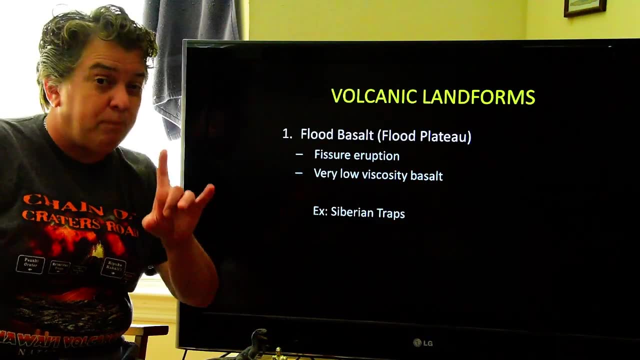 Are you talking about the biggest volume erupted? Are you talking about the biggest explosion, The biggest impact on people? You know there's different ways of looking at that, But if you're looking at the biggest volume of material erupted, then it is. 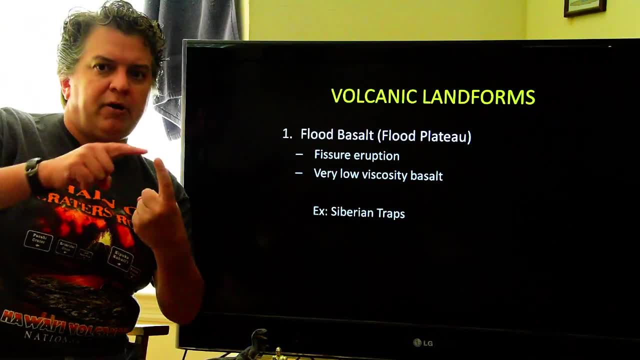 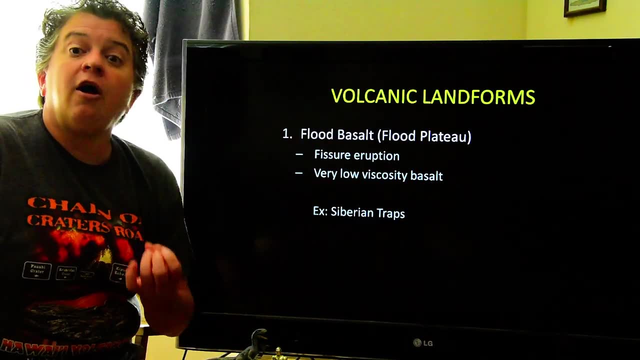 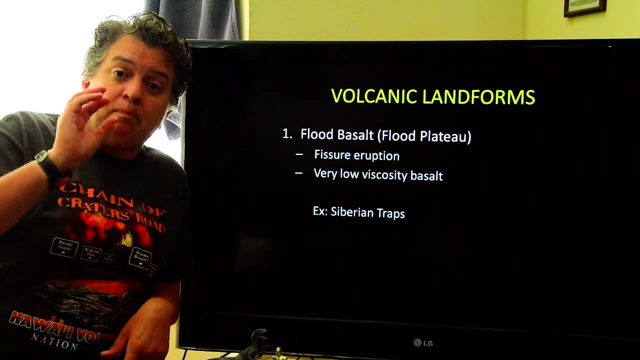 flood basalts. So let's look at our three Vs. This is going to be very large volume, very low viscosity and low volatiles. It's not explosive, right, It's just lava flows And when it comes to big fissure eruptions. 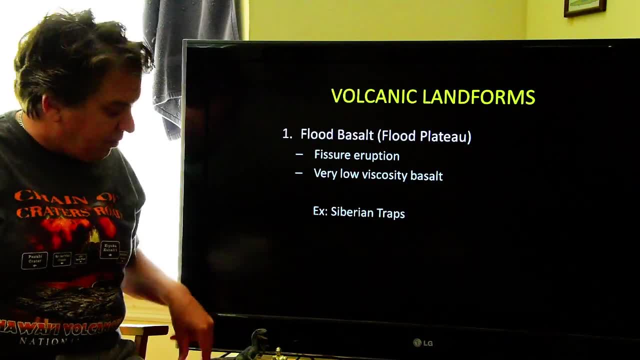 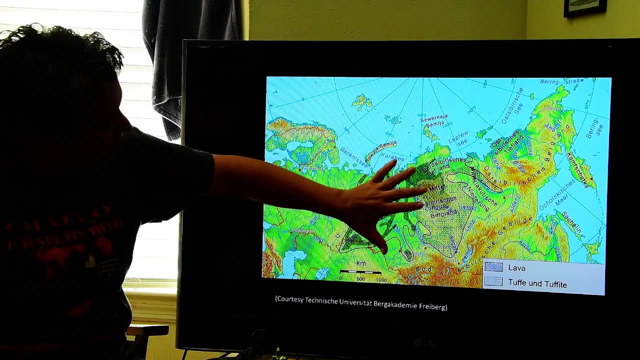 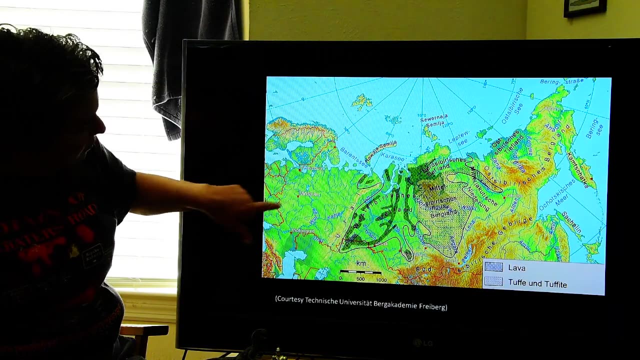 big flood, basalt eruptions. a great example is the Siberian Traps, And so just to get you oriented here, this is Asia, This is Scandinavia, So there's like Norway, Sweden, Finland, There's Moscow. 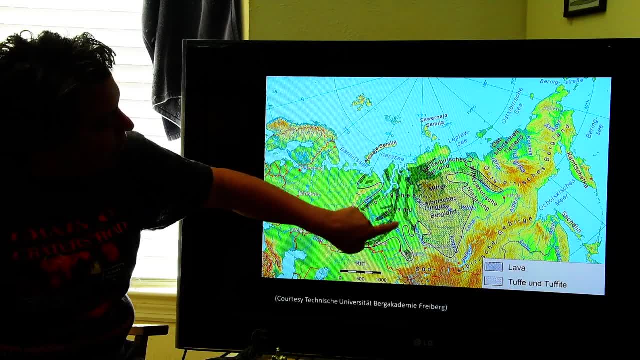 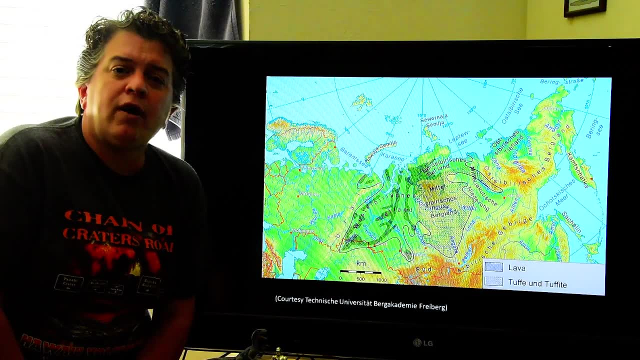 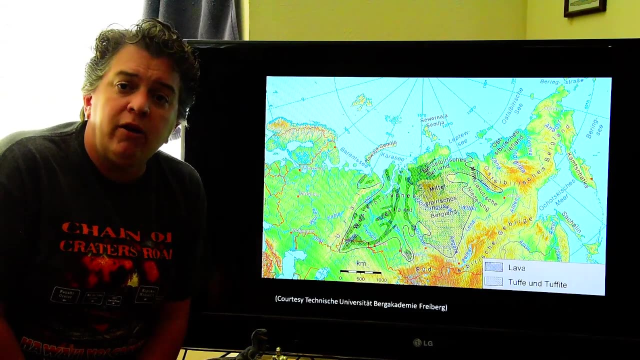 This black line outlines all the land covered when the Siberian Traps erupted. About 800,000 cubic miles of lava was erupted and that covered about 1.5 million square miles, And that's pretty much the Imagine the entire United States. 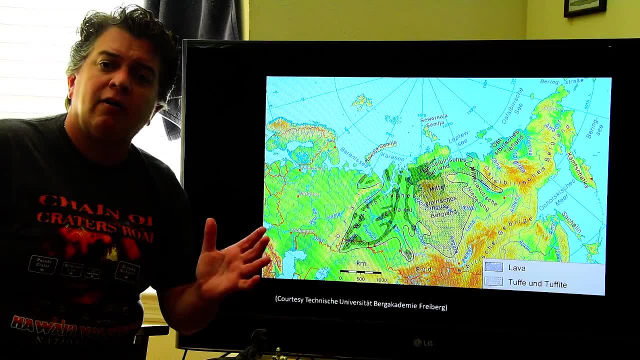 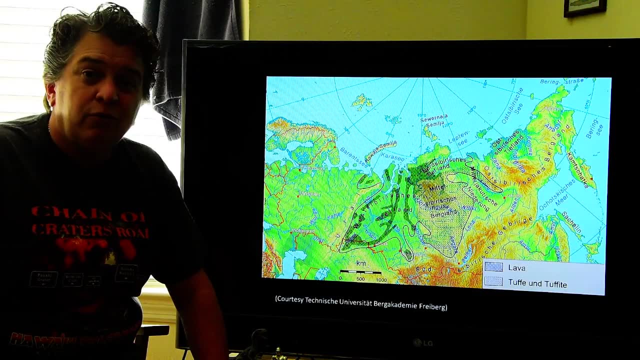 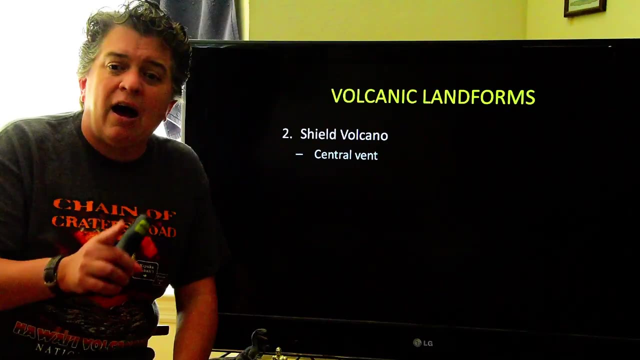 west of the Mississippi being covered by lava. That's about how much land area the Siberian Traps covered. So we're talking a huge part of land. So those are very big eruptions But they don't form mountains, okay. So you're not going to be talking about. 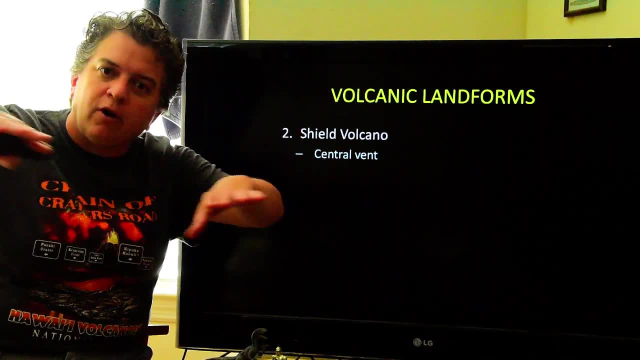 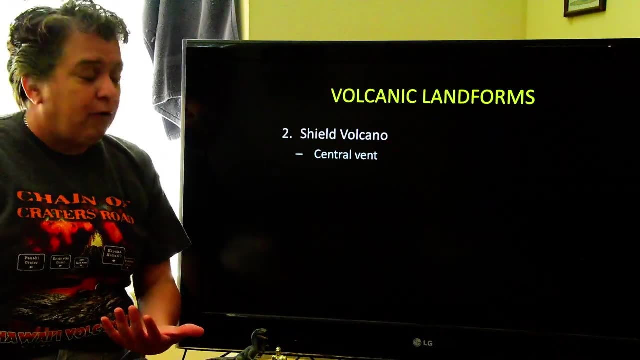 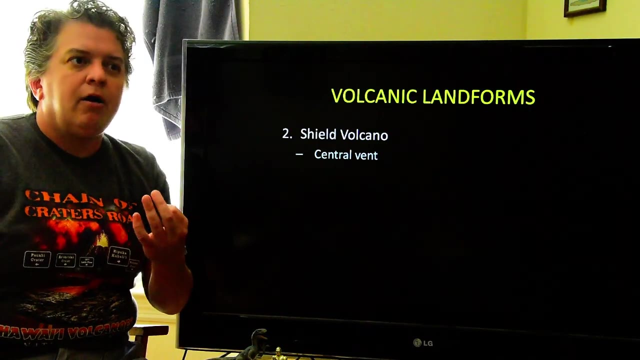 a volcanic mountain there. That's why it's called a plateau. It's going to form this like nice flat area, All right. Another type of volcanic landform that you can get is called a shield volcano, And a shield volcano is similar but different.